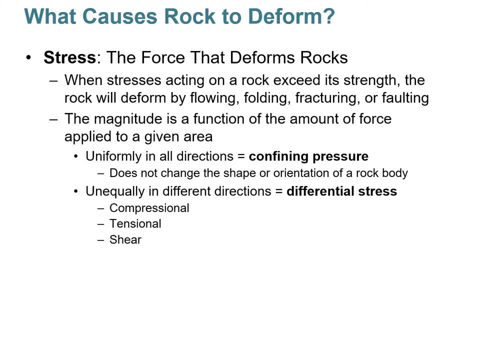 kind of impinging on a rock and it exceeds its strength, the rock will deform. And it'll deform by any of these four F words: flowing, folding, fracturing or faulting. So the magnitude of the deformation is a function of the amount of force applied to a given area of the rock. 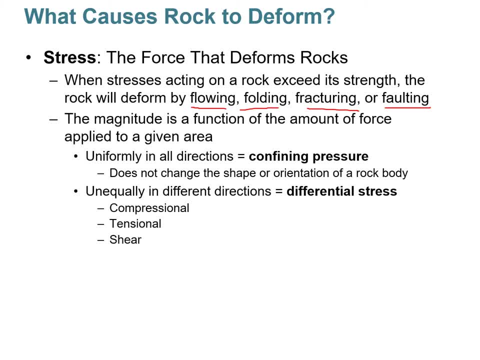 If the forces being applied to the rock are equal in all directions, we call that confining pressure. And if they're unequal, meaning that the forces are kind of coming at the rock in different directions, we call that differential stress. And there's three types. There's compressional. 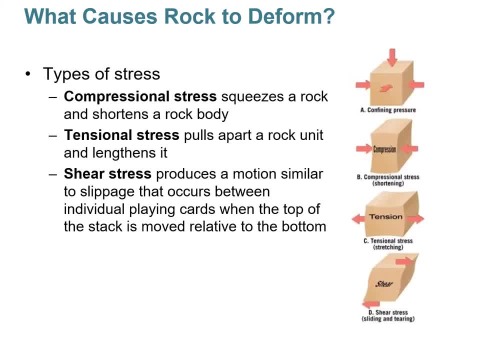 tensional and shear. So here are the different types. This is confining pressure. This is analogous to jumping into a pool and swimming to the bottom of the pool. You know you have to kind of yawn or pinch your nose shut and blow to equalize that pressure. That's because 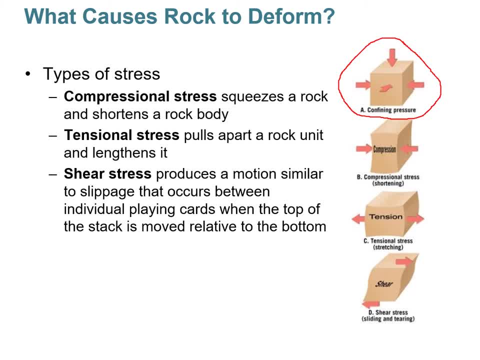 you're under increased pressure, The weight of the water column is applying forces to your body equal in all directions. Okay, Compressional stress, which is pictured here. this is where a rock is squeezed, And so imagine, this used to be a cube like you see up here. It's the 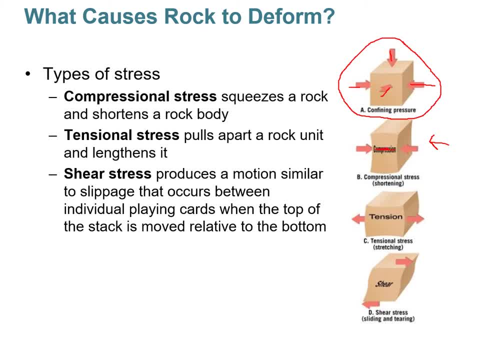 direction of the rock is shortened in this direction and elongated in this one. Okay, Tensional stress does the opposite. Tensional is pulling apart. That's the stress. Okay, So you actually lengthen the rock in this direction and shorten it in this direction And then shear. 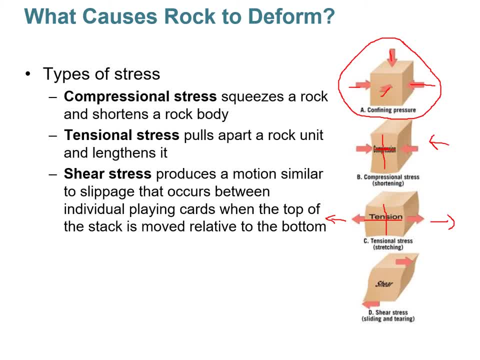 stress. this is where you have stress forces being pushed into opposite directions, And the best way to visualize this right here is: imagine a deck of cards. You put your hand on the top of the deck and you push the deck this way, And then you push the deck this way, And then you push the deck this. 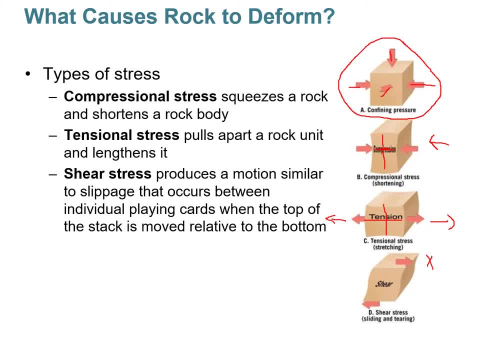 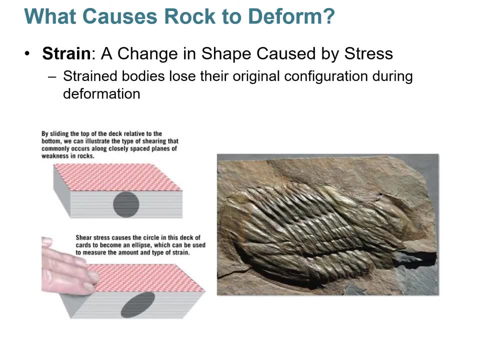 way The cards down here won't move, And then the cards up here will move in that direction and create this unusual shape. Okay, And that's shear stress. In fact here's a picture. You can visualize it kind of nicely right here. So strain is a measure of how much the rock body has kind of moved. Okay, 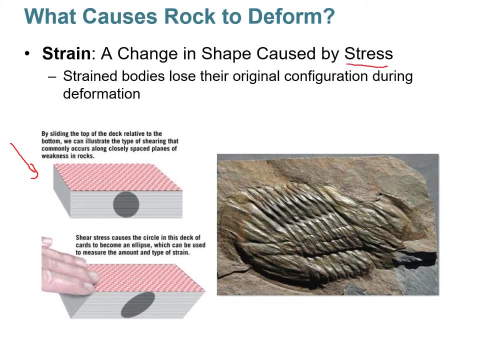 So a change in shape that's caused by stress. So you can measure strain like, especially if you have a fossil in it, that's a trilobite. They don't look like this. This has been stretched and kind of pulled apart because of shear stress And you can measure how much a rock's been. 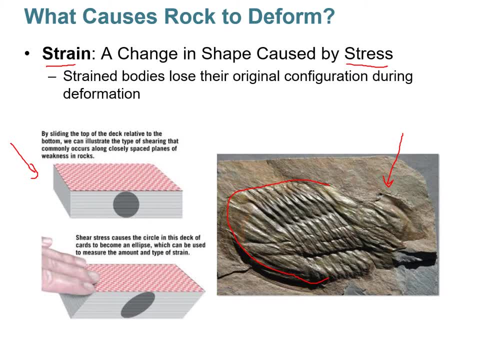 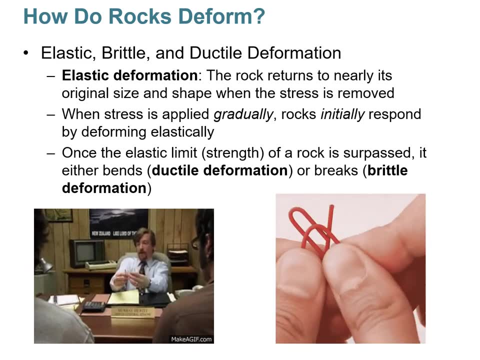 shortened or lengthened as a result of stress. Okay, So there are three types of deformation. Elastic deformation is when the rock returns to its original size and shape. Imagine a rubber band. So like: start expanding that rubber band out bigger and bigger and then letting it go. The 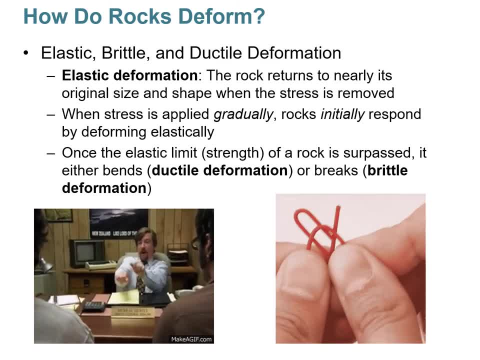 rubber band will return to its original shape and size after the stress is removed, Right. But if you continually pull that rubber band out really far and far, it'll eventually snap Right And then turns into a weird rubber noodle. That's called brittle deformation. That is when a material kind 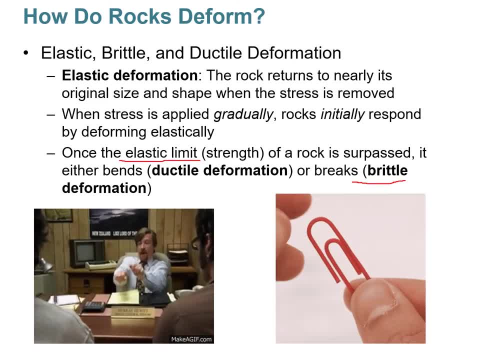 of once you exceed its alignment, you're going to have a rubber band that's going to be able to break. So if you exceed the elastic limit, so the rubber band's elastic limit, then the rubber band will brittly deform and it'll snap, Kind of like this cool dude is snapping a pencil. There you go. 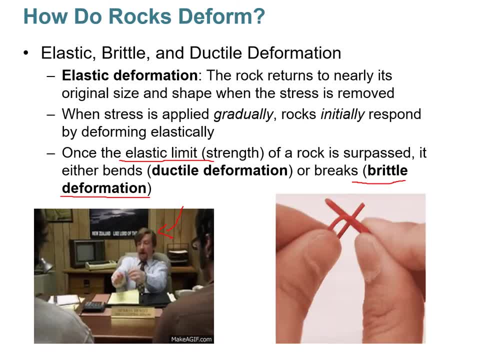 New Zealand. That's brittle deformation. You're changing the shape of whatever it is. you're putting stress on forever, Okay, And breaking it in a kind of rigid fashion. But you can also exceed the elastic limit of a rock or any other substance, Right. So if you exceed the elastic limit of a rock or any, 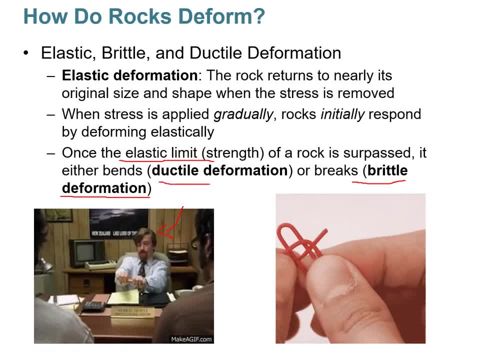 other substance, you're going to have a rubber band that's going to be able to break Right. So if you exceed the elastic limit of a rock or any other substance and it can bend- and we call that ductile deformation, And the example here is a paperclip kind of being bent into a new shape- 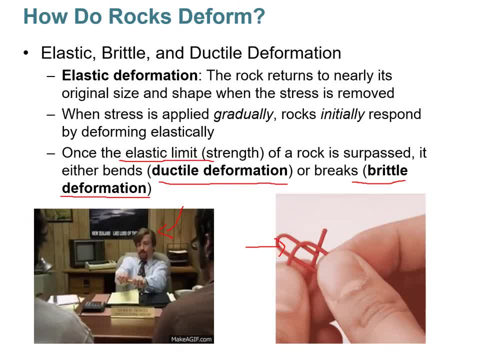 like a pretzel or something. Okay, And so when stress is applied gradually, rocks initially deform elastically, But over time you can exceed the elastic limit And then it, and then it kind of falls into the realm of either ductile or brittle defomation. So here's an example of how to ediyorum. 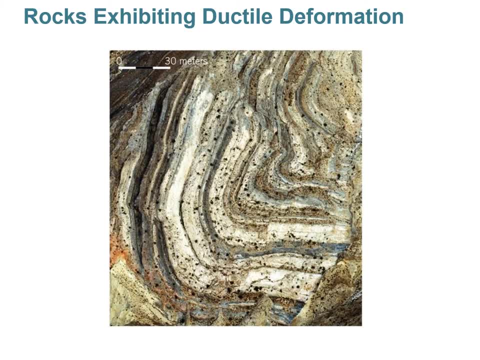 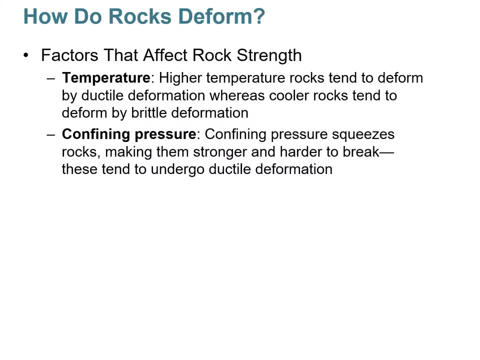 a rock when you're bending into it, Mark cliff, of a rock that was ductilely deformed because you don't see a break. you just see kind of like a fold in these layers here. So there are a number of factors that affect a rock's strength and then that will determine. 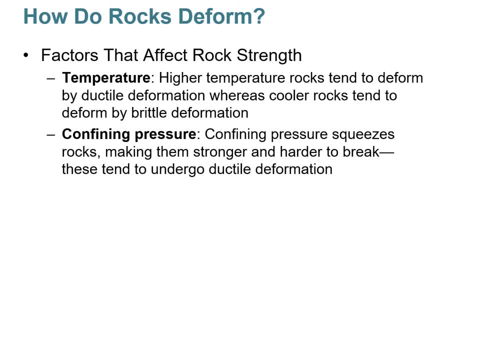 whether a rock will deform brittly or ductilely, and one of the most important factors is temperature: Higher temperature or an environment with really high temperature. where the rocks are under high temperature, they tend to deform by ductile deformation, whereas if you're 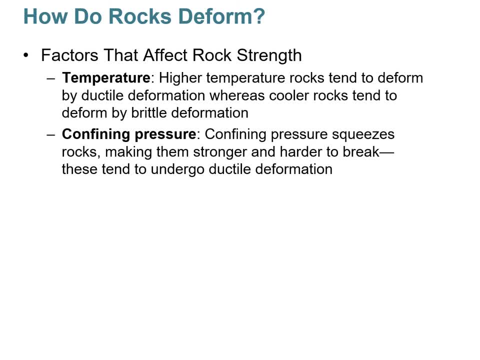 in a low temperature environment, typically closer to the surface of the earth, rocks will brittly deform. Another variable in this is pressure, and confining pressure kind of squeezes rocks and makes the kind of small spaces in between them disappear and that makes them stronger. 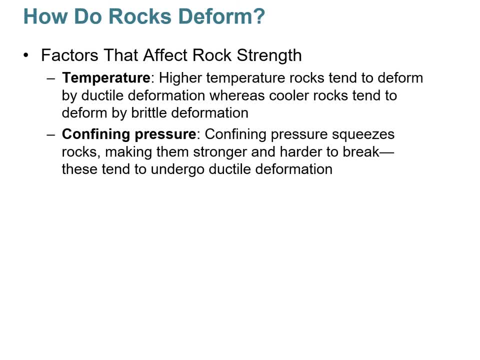 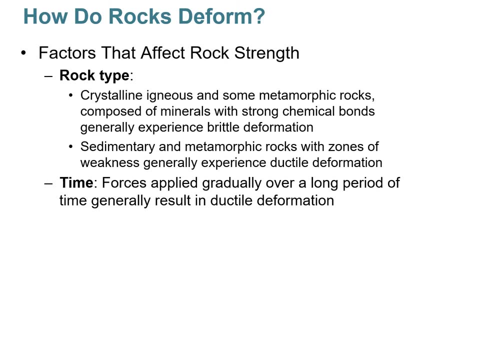 and harder to break, So these tend to undergo ductile deformation. So that means the rock will deform, But that's usually deep in the ground within the crust. Rock type is also important If you have crystalline, igneous and some metamorphic rocks, they're typically composed. 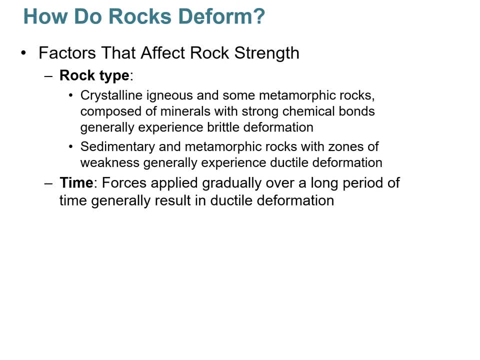 of minerals that have strong chemical bonds and they're kind of interwoven together, So they will generally experience brittle deformation. but it really depends on other factors like temperature and pressure. Sedimentary rocks and metamorphic rocks tend to deform. So if you have crystalline, igneous and some metamorphic rocks with zones of weakness, 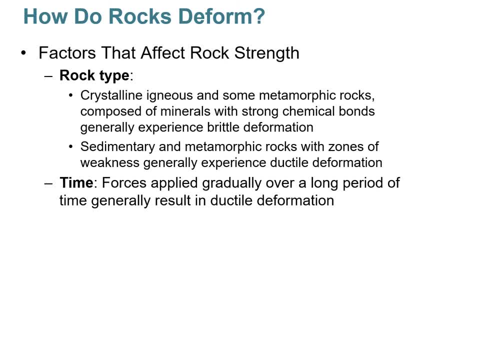 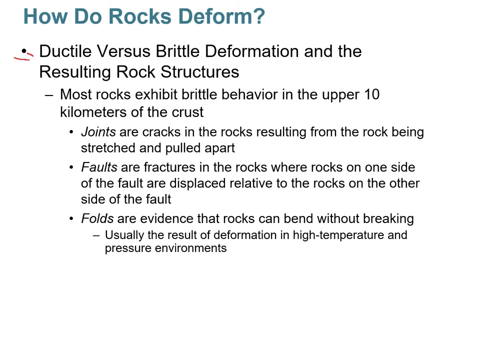 or different types of foliation, they'll exhibit ductile deformation because they're weaker. And then the last factor is time. So if you apply stress and these forces gradually over a long period of time, that will result in ductile deformation. So how can you know what environments would you typically see ductile or brittle deformation? 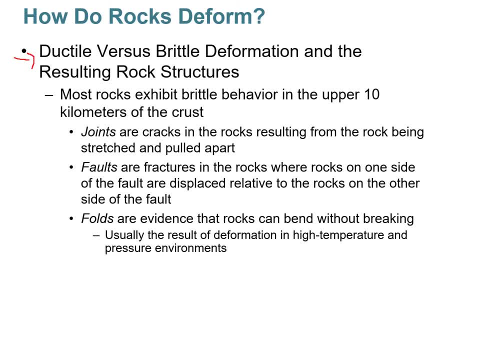 Well, you know there's a lot of different ways to see ductile deformation. There's a lot of different ways to see ductile deformation. You know you can look at rock deformation. what will occur more often? Well, if you're in the upper ten kilometers of the crust, most rocks will exhibit brittle. 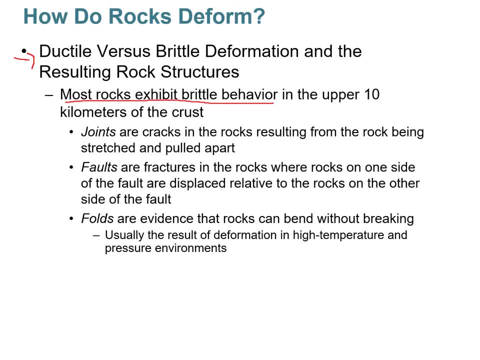 behavior So they'll start to kind of break or form faults. Okay, Some of that brittle behavior are joints. Joints are kind of cracks from rock being kind of stretched or pulled apart. A lot of times that's just being at the surface. 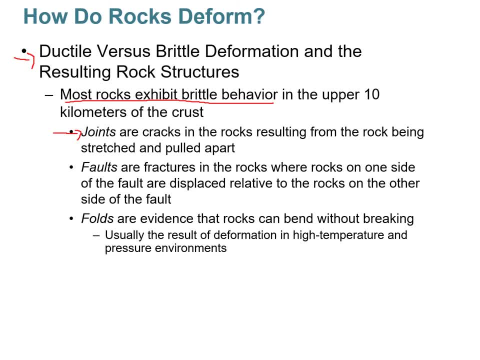 Rocks form under tremendous pressure deep under the ground. So they'll start to break or form faults. the ground, and when you have uplift and erosion exposing these kind of deep rocks, they kind of expand outwards and they'll form these parallel, joint cracks. um, faults can also form. that's a. 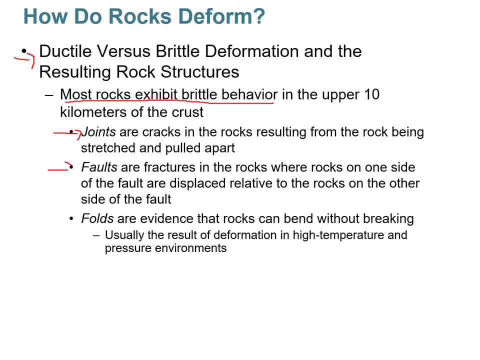 type of brittle, brittle behavior, and these are just fractures in the rock where there's displacement- okay. and then folds are when rocks ductily deform- okay, that's when rocks bend without breaking, and that typically happens, uh, in high temperature and high pressure environments, which means that's. 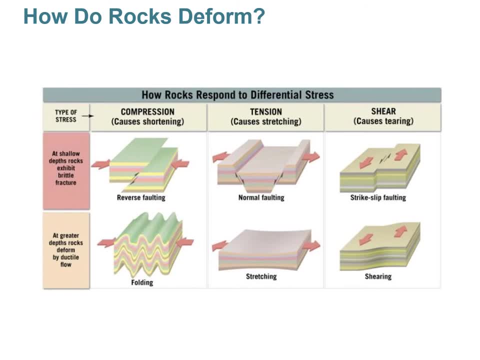 deep underground. so here are the, the kind of six examples. um, here are the different stresses, here's compression, tension and shear, and then in this row here this is the examples of brittle deformation, and then down here are the examples of ductile deformation. so if you have compressive forces, 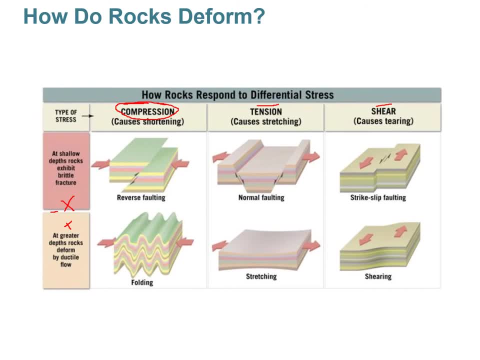 okay, as if a rock was in a vice. if the rocks deform brittlely, you'll form a reverse fault. if they, uh, deform ductily, you'll get folding. okay, and so these rocks start to fold. if there's tensional stress or pulling apart, um brittle behavior will. 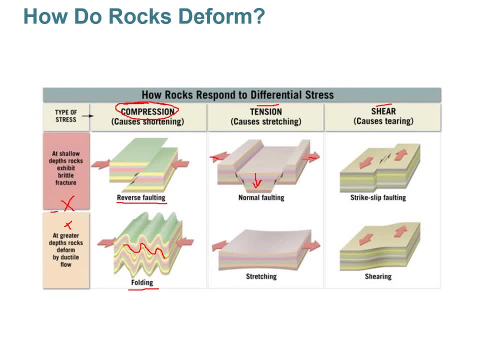 create normal faults where this block kind of falls downwards and these two go up. okay, um, in a ductile deformation scenario you get stretching, so you get thinning of these rocks here. then if you have shear stress, the brittle deformational example here is a strike slip. 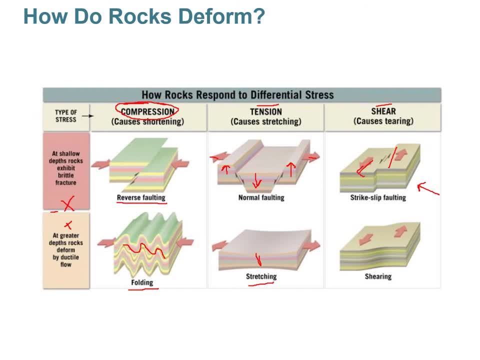 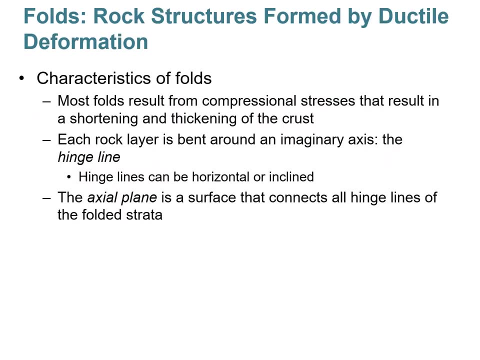 fault where two blocks move in the opposite direction creates a fault, and then here you'll have stretching. okay, so let's talk about ductile deformation. uh, some examples of this. so folds- most folds- result from compressional stress, so that involves shortening, uh, the crust, and thickening. 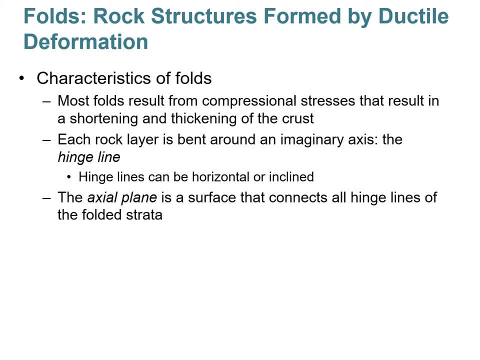 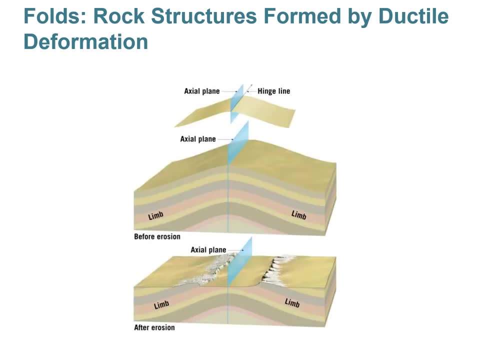 it, and then the rock layers typically bend around what we refer to as a hinge line, which is an imaginary axis that cuts right through the center of the fold. and hinge lines can be horizontal to the surface of the earth or they can be inclined, and then the axial plane is this plane right here. 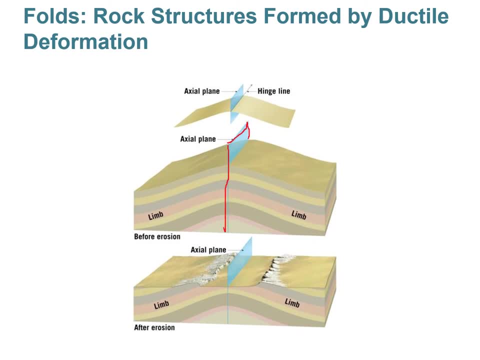 that goes right through the center of the fold. okay, so that's the center of the fold. these are the two limbs on either side of the fold, and then this here: this line here would be the hinge line. okay, and typically when this compressive action occurs, then you'll have erosion and see here these would be exposed or outcropped. 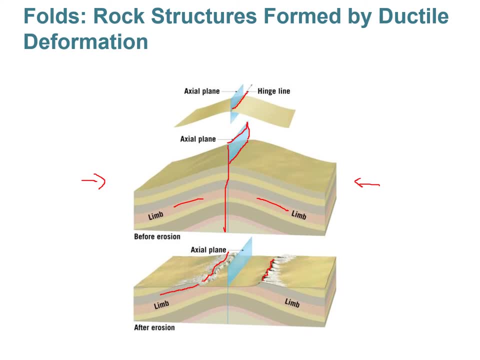 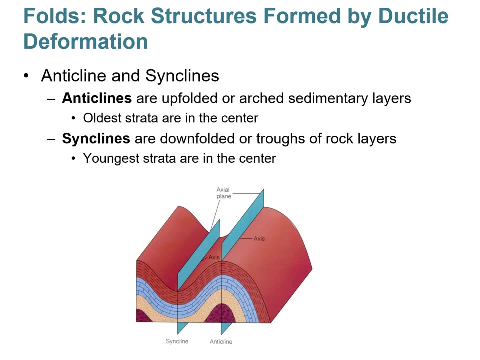 rocks and you can see they kind of dip downwards into the earth. so there are two types of folds: anticlines and synclines. anticlines are up folded or arched sedimentary rocks. so that would be this right here. that would be an anticline. okay, um, and what you notice about anticline is after: 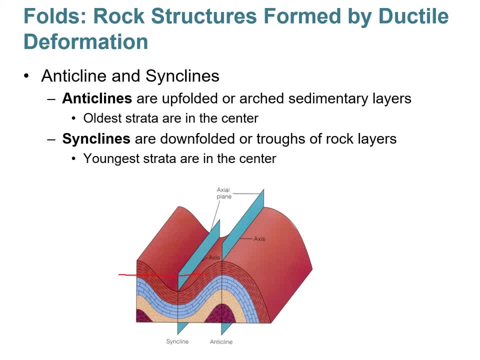 erosion has taken place. so let's imagine you kind of cut- you know, an erosive layer here, these older rocks, because they're up, arched, they're pushed upwards. you'll find oldest rock near the center- i have another image that shows this a little better- and then typically together these folds occur. together you'll have 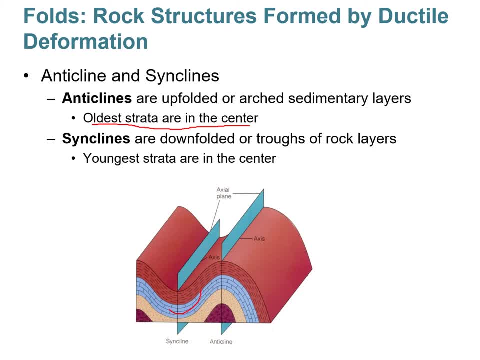 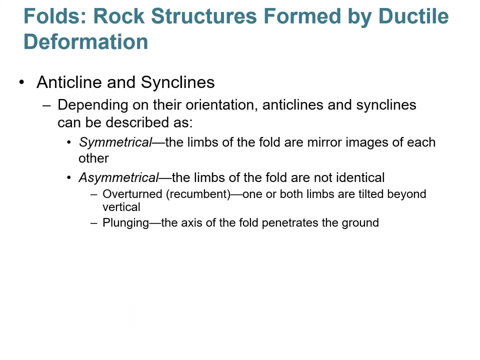 synclined folds. so these are these downwarped folds here. so this would be a synclined fold here. so you see how these rock layers are kind of bent downwards and here, if you create that erosive surface, the youngest layers will be at the center. you'll see that, i guess, in the next slide then. 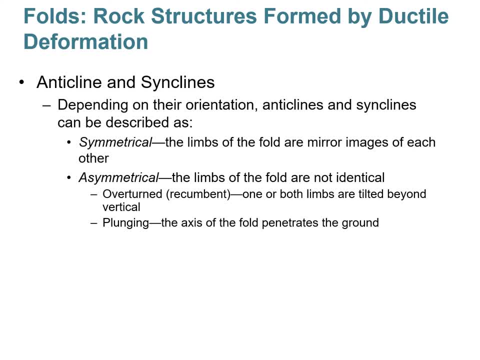 depending on the orientation. if you're not familiar with this, you'll see that the anticline and synthesize pairs can either be symmetrical or asymmetrical, okay, and the hinge line can actually plunge within the earth, and we'll take a look at that. let's go right to the image, because it's so much easier showing you. 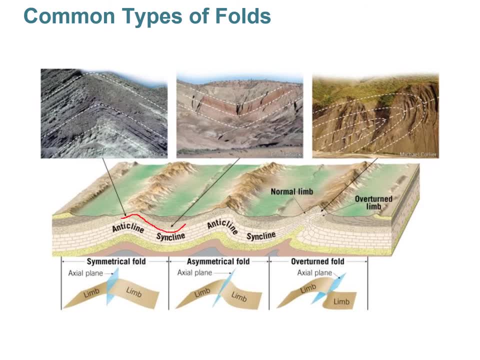 this. so here's an anticline and syncline pair. these are symmetrical folds. and then you see, here the oldest layers are down, here the oldest rock. so in an anticline, after some erosion, these older layers get exposed at the surface. so that's why you typically see: 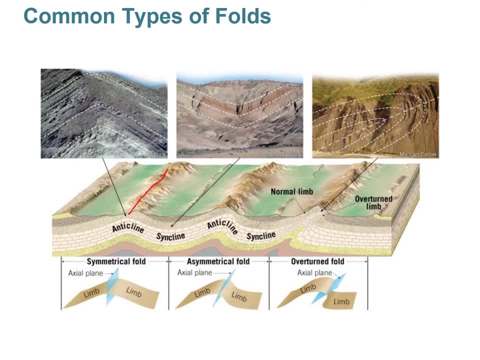 at the center of an anticline. you see older rocks exposed at the surface at a syncline, because it's down warping. younger rocks are preserved at the center of the fold. okay, this is what they look like in cross section. okay, and the way i like to remember this anticline starts with a, and that's. 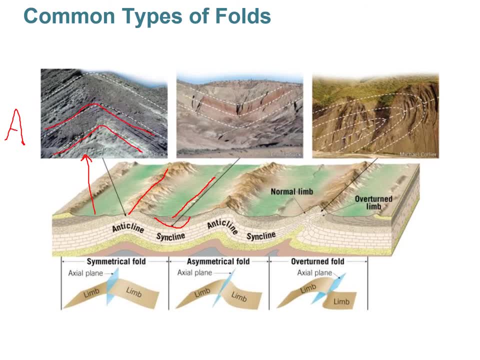 what the rock layers look like: up arched rocks like this, a for anticline. and then when you see this here, this is in the field, live in action, here's a syncline- and you get that down, folded, fold like this: okay, now, not everything's easy and perfect. uh, sometimes these are, these are. 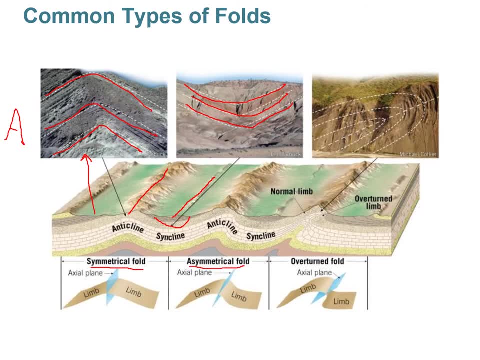 symmetrical folds. sometimes you can have asymmetrical folds, and with asymmetrical folds the axial plane is tilted, it's not straight up and down. so what happens is one limb ends up being longer than the other limb. okay, and sometimes it's. this is so, uh, compression can be so great. 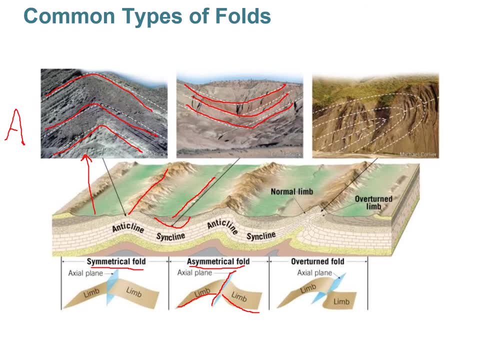 that the the fold itself can overturn and this is very confusing and this is what it would look like in the field. so this rocky, this rock unit, which is the youngest one, has overturned and kind of overturned underneath some older rock units over here. it's almost like a crash, crashing wave. do you see this kind of a wave? 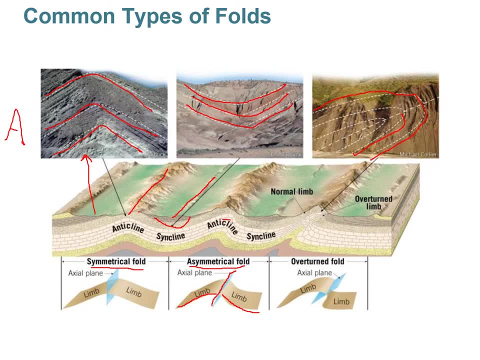 approaching and then crashing over. here would be the overturned limb. and then you see here this axial plane kind of almost becomes horizontal. okay, it's like tilted and this limb is thrust over to the other limb. that would be an overturned limb. so if you can get kind of confusing, structural geologists have 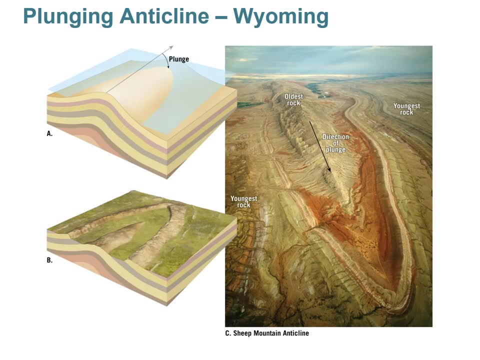 difficult job. and then the the hinged line is not always like right on, like parallel with the ground surface. sometimes they can point downwards, so they can. this is called a plunging fold, so the hinge line plunges down into the earth, and so what you see here, this is a plunging 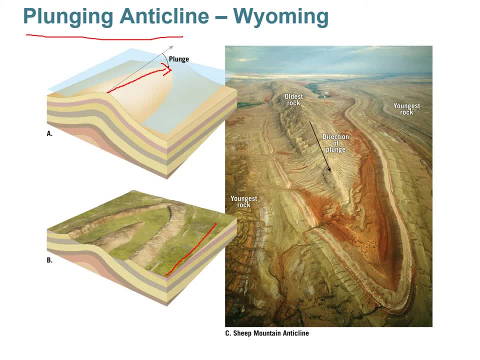 anticlockwise, and this is what you see here. this is a plunging anticlockwise. here's the example in Wyoming. in fact, you can see a lot of this if you go, if you go on like Google Earth, go to satellite images, go out to Western PA. 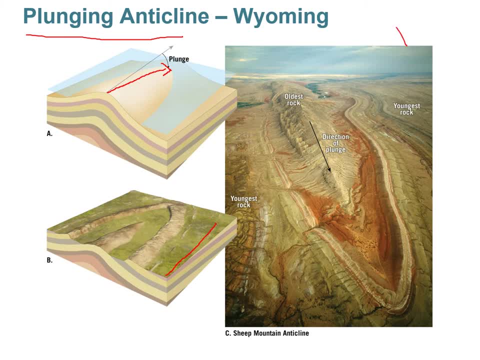 and you'll see this pattern in in the exposed mountains there in the valley in range province. but but this is what you would see. this is what the outcrop rocks would look like with this kind of parabolic shape here, and then this older rock that's that's up arched because it's a sink line, is exposed here. but 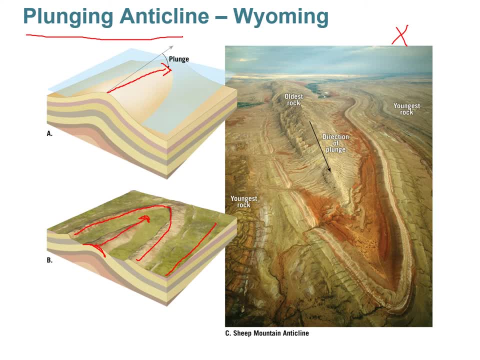 then it kind of just disappears into the ground, okay, and that's because of that this is an inclined anticline, so that the hinge line is pointing downwards and so the deeper rocks just kind of disappear as the fold moves in, and that's why you get that kind of exposed parabolic outcrop of rock. it's 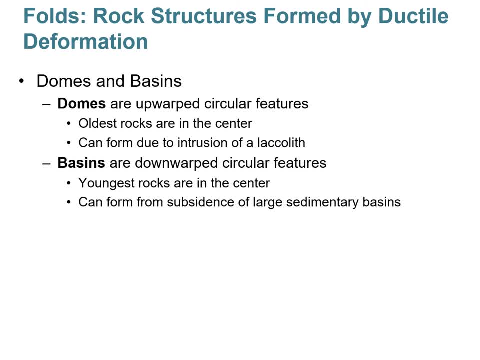 really interesting. there are also similar other structures created by ductal deformation: domes and basins. domes are up warped circular features where the oldest rocks are in the center, and think of like the bowl you would have or you'd have like a bowl of cereal. now flip that. 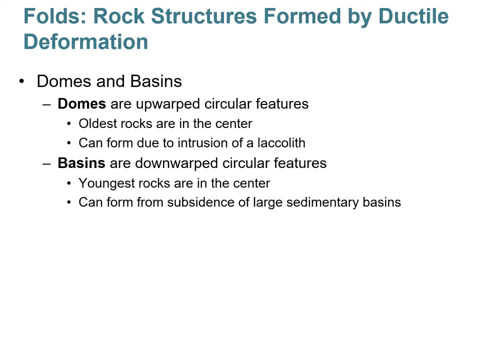 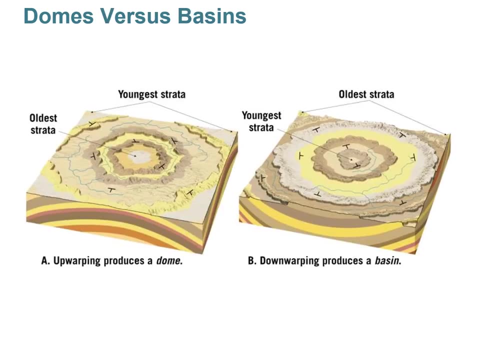 bowl around and that would be a dome type shape, and then basins, like how you would have a regular bowl of cereal- the bowl itself, not the cereal- and that those are down warped circular features, and the youngest rocks are typically at the center. so here's your dome. 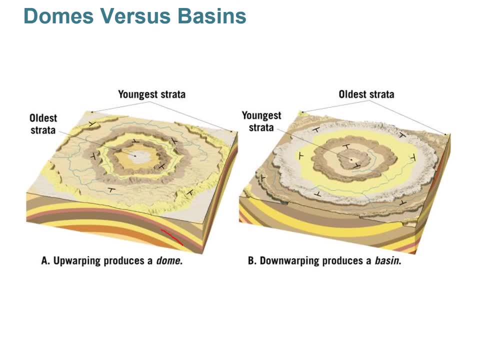 okay. so you see that here are the up warped circular features, and after erosion you'll have exposed older rocks at the center, and as you travel outwards you run into younger and younger rocks outcropped in circles surrounding it. and then here's your basin and this is the octa. it's almost like someone put their 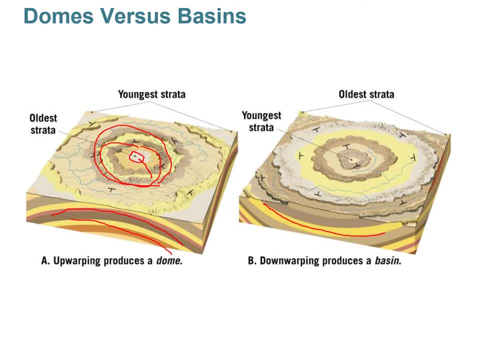 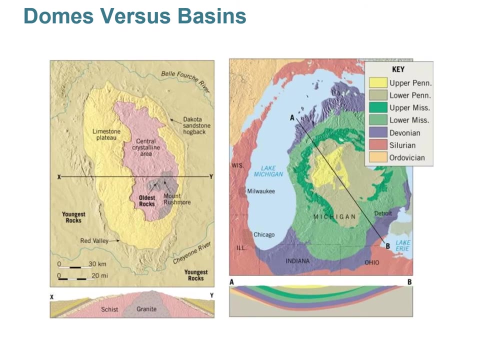 finger in the center here and just push downwards and then everything kind of buckled in a concave upward direction fashion. and this is real. we see places here in the United States that show these structural features. if you've ever been to South Dakota to see Mount Rushmore. 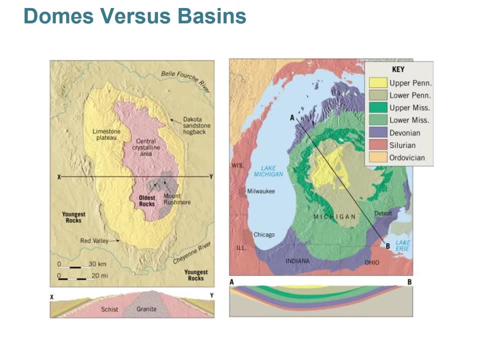 Mount Rushmore is a dome. you see here, this is a cross-section from X to Y, so this is the cross-section of that area and what you see here, see this: this is a limestone that's outcropped here. then it kind of disappears, but you see it on the 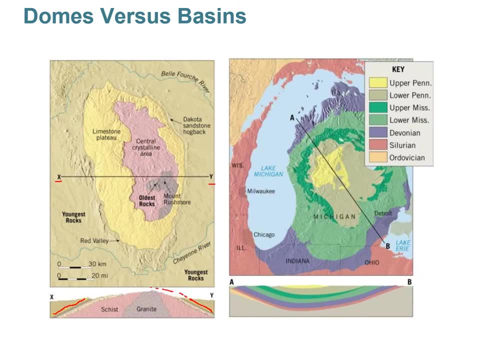 other side at some. at one point they used to be connected over like this and that creates that dome. but erosion has kind of since taken that over, and at the center of this dome is the exposed granite right and that's where they've carved those famous American icons onto the granite. 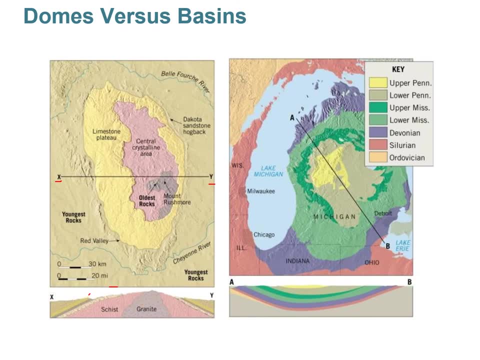 ok, then if we go to the Michigan Peninsula, you can see here this is the basin, and so here at the center of the Michigan Peninsula, you have the youngest rocks exposed here and then, in the circular fashion, all the rocks outcropped further and further. you go away from this basin. 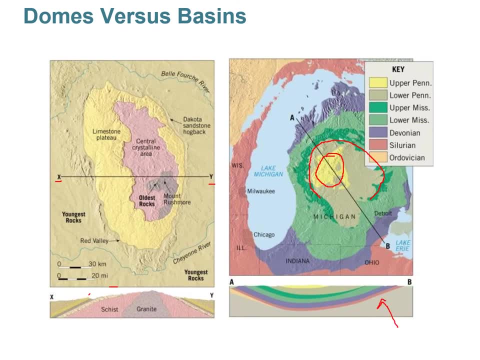 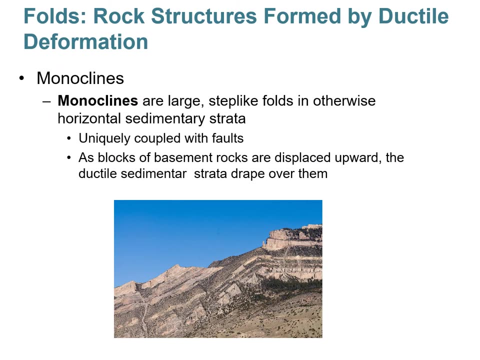 ok, so here's that underground kind of structure, the the bowl, so to speak. here's the upside-down bowl. then there's another structure that forms from ductal dust. The bottom of the bowl is the basement, and in the middle there's the top of the bowl. 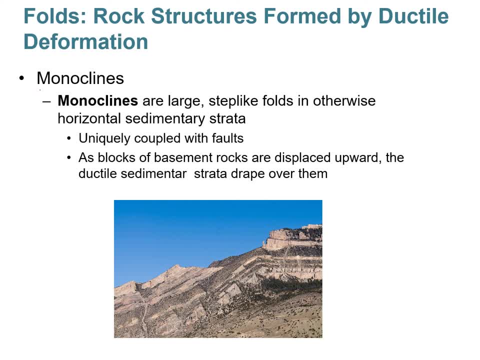 top of the bowl is the bottom of the bowl. deformation and it's called a monocline, and monoclines are step-like folds, okay, and typically occurs in horizontal sedimentary strata that overs, that kind of sits on top of more crystalline rocks, and so you see, here this is kind of. 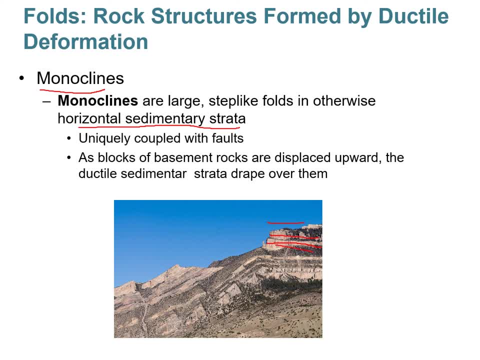 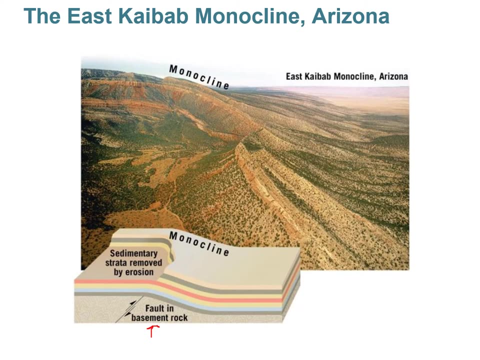 horizontal sedimentary rocks right, and then there's this kind of down fall folded rocks right here, so it's almost like a one limb that's kind of folded downward like this. okay, so, as basement rocks readily deform, maybe create this fault, this pushes these once horizontal sedimentary rocks upwards and then it. 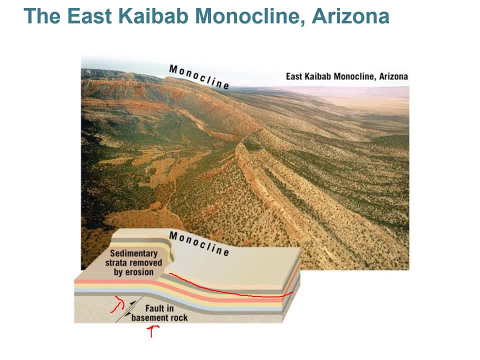 creates that gentle fold that you see in a monocline, and a lot of times, after there's some erosion, what you're left behind with is kind of this wall of kind of dipping sedimentary rocks. this is in Arizona, here's the East Kaibab monocline, and a lot of these monoclines were presented. 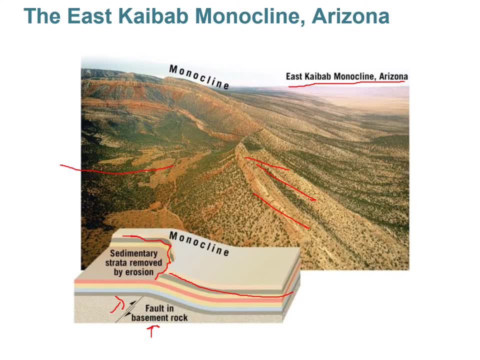 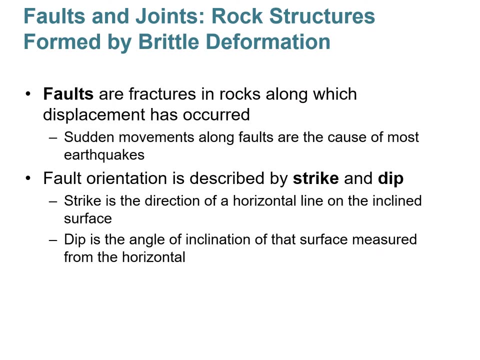 huge problems for people kind of settling out in the American West. it's hard to traverse. okay, let's talk about brittle deformation now. and brittle deformation are when rocks kind of fracture and displacement has occurred and we've kind of talked about this already along those faults. that's where 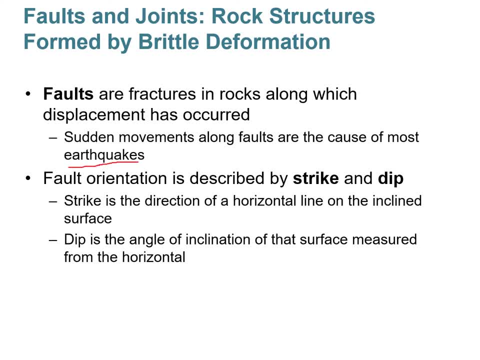 earthquakes are created, and so the orientation of the fault is described by strike and dip. okay, the strike is the direction of a horizontal line on the inclined surface. okay, now, I know it's gonna be hard to draw, so it just imagine this is three-dimensional. oh god, okay, that's not too bad. that's not too bad, okay, so let's pretend the 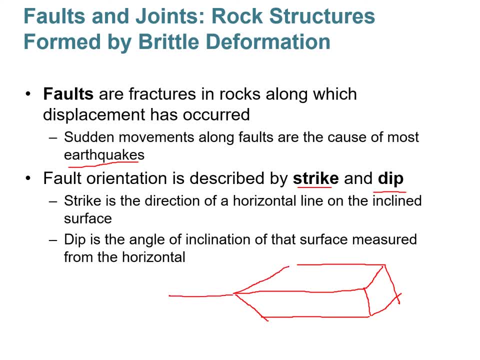 fault surface is here. here's the fault, and then this is kind of two rock blocks here. this here is the fault surface, and then this here would be the strike. this is on the horizontal line, all right, so this is the strike, here s for strike, and then this is the fault surface. the dip would. 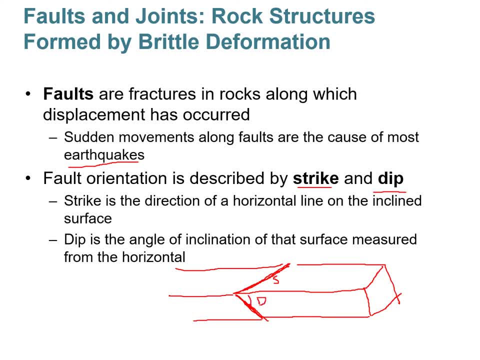 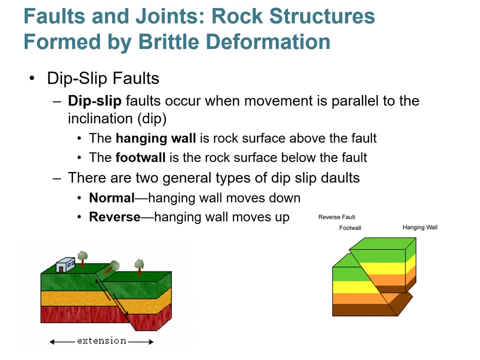 be this angle here, so that's the okay. so the dip is the angle of inclination from the fault surface. so here's a fault surface and it's inclined from this angle, from the horizontal. I'm actually pretty impressed with that drawing. okay, so let's show you some examples. oh, we got gifts. dip slip faults occur when 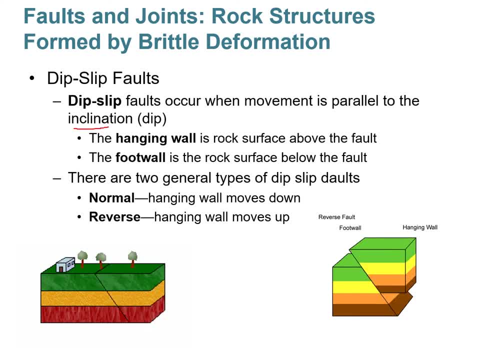 there's movement that's parallel to the inclination or the dip, and there's two features: a hanging wall and a foot wall. the hanging wall is a rock surface above the fault and the foot walls below the fault. so here this. here is the foot wall. we'll put an F here, okay. 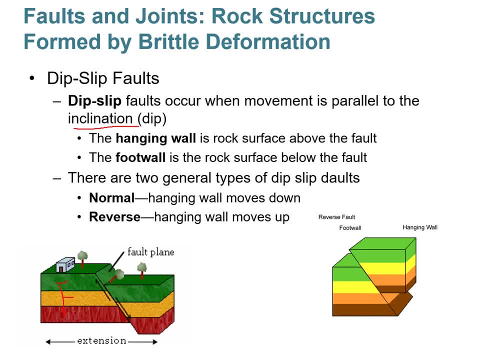 the foot wall. I'd like to imagine I'm a giant and put my foot here to tie my shoe. so this is the foot wall block here, and this is H for the hanging wall block, okay. and over here, this example: this is the foot wall, okay. and then this is the. 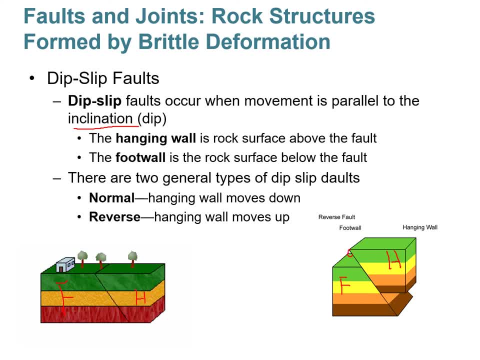 hanging wall and I like to remember the hanging wall because, like see that you can kind of hang off of this sharp edge over here. I don't know that's how I remember it anyways. so there's two types of dip slip faults, because you can have motion in two ways. you can have normal where the hanging 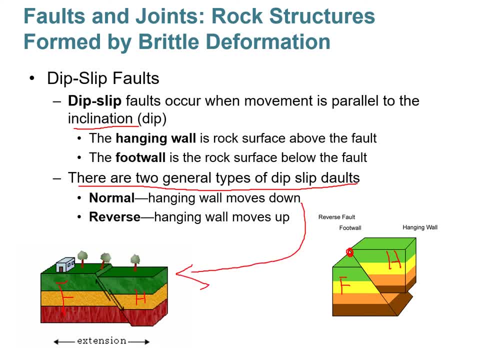 wall moves down, and that's this example over here. you see that H moves down, the hanging wall moves down, and then reverse. where the hanging wall moves up- and that's this over here- see the H kind of moves up. that's the hanging wall that moves up. that's reverse, and this one's normal and for normal. okay, so let's take 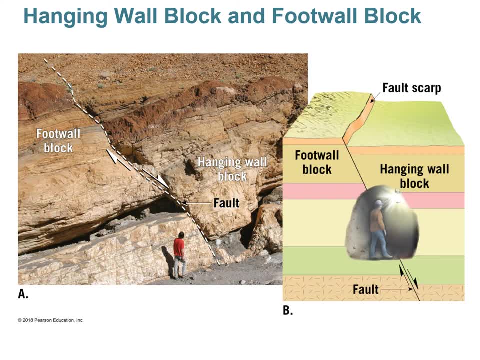 a look at this. let's see if can you guess what? this is? all right, if this is the foot wall, right, you can put your foot on it. here's the fault plane. this is the strike of the fault. here's the hanging wall block right. what kind of fault is this? you said normal. then you are correct. yes. 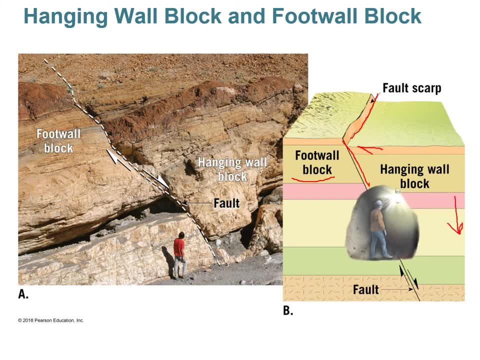 it's a normal fault. the hanging wall moves down. okay, you can see, see these layers, how there's displacement. this pink layer used to be aligned with this pink layer, but because of the movement, you're no longer aligned. and when you go out into the real world, this is what you see. 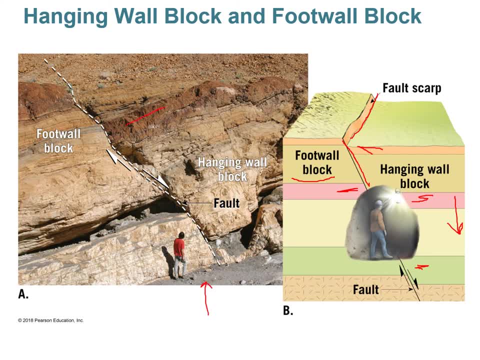 you can see these layers over here and this is what I mean by hanging wall block. so the normal fault here is here. you can see any of the falls: the Tanner and some fell over there. so here are some. this is a rock unit- clearly the same rock unit- over here, and they've been displaced. you can measure that. 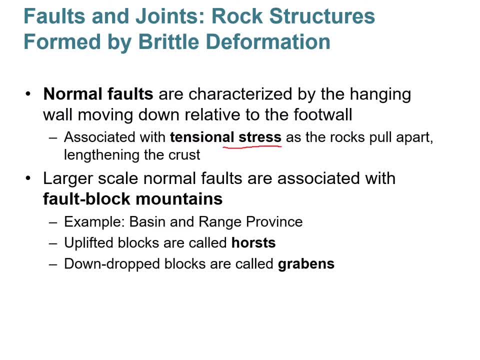 displacement. and so here, what you have here, this is a foot wall block. there's a hanging wall block. this is also a normal fault, And when you have this occur in a large scale on a tectonic plate, we call that fault, block mountain, So you can create an area that has kind of mountain ranges as a result of tensional stress. 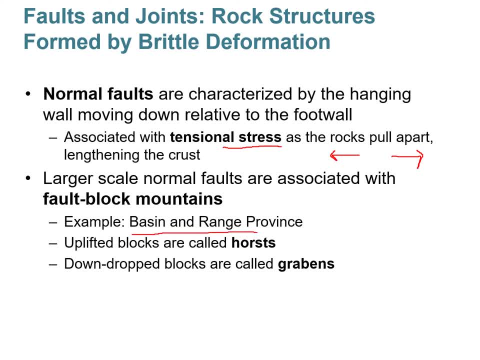 And the best example of this here in the US is the Basin and Range Province, And what you see is uplifted blocks- We call those horse- and down drop blocks, We call them grobbins. All right, So here's your normal fault. 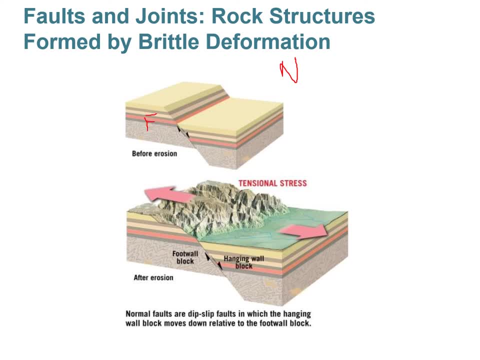 And here, right, your foot wall moves up and your hanging wall moves down, And here you get a normal fault. And then so what happens is, because this foot wall moves up and the hanging wall moves down, you're kind of exposing all these older rocks and creating a range over here. 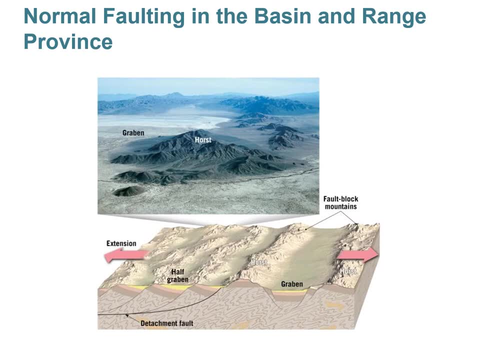 And then this is the Basin and Range Province. So here you got range, basin, range, basin, range, basin, And it goes on forever, Like the entire state of Nevada, And the entire state of Nevada is made up of these kind of north-south trending ranges and valleys. 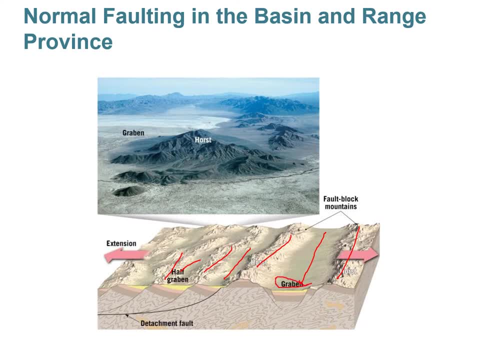 Okay, So we call this a grobbin here, this low-lying area that's filling up with sediment, And these would be the horse, And that's the result of tensional stress or extension. Okay, Reverse faults. they're associated with compressional stress. 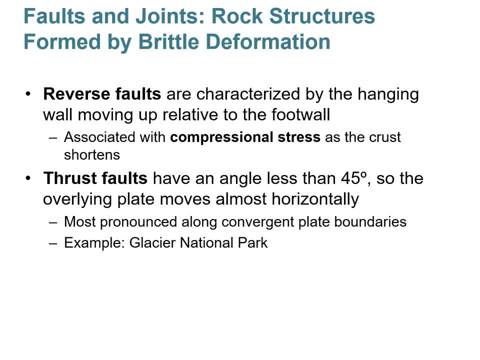 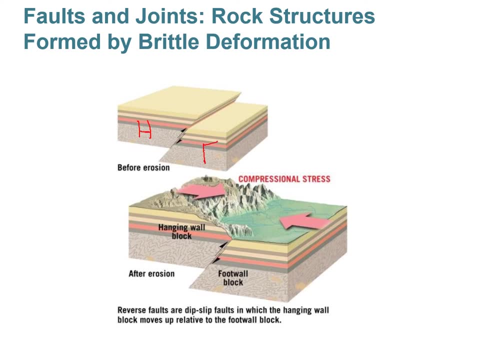 And these can create what we refer to as thrust faults. And a great example: This is at Glacier National Park and these occur at convergent plate boundaries. All right, So here, hanging wall moves up, foot wall moves down, F moves down. 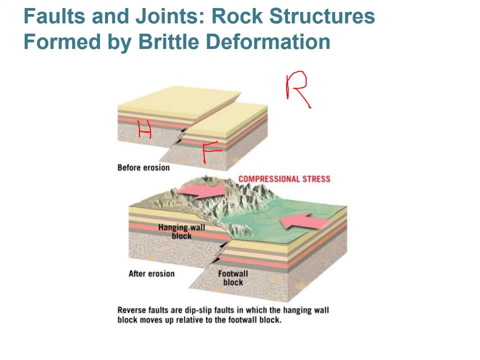 And then so this is a reverse fault. And so what happens? you also create mountains as well, because you're kind of pushing up older rocks upwards and this is going downwards, And then over here you have some mountains, and here's some good example of the formation of a low angle thrust fault here. 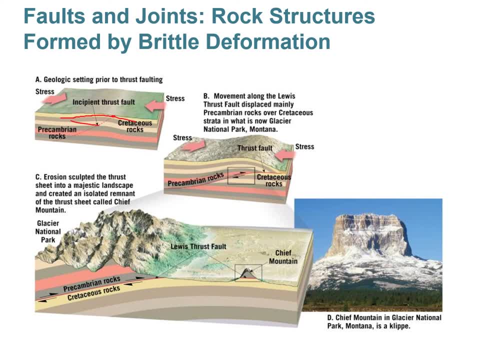 So all these rocks kind of were Horizontal, but then they started compressing right Here's the direction of stress. And um, Oh, I can't get the eraser. Okay, There we go. Um, and then this fault forms right here. 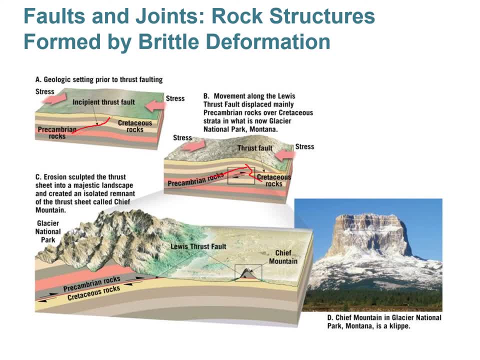 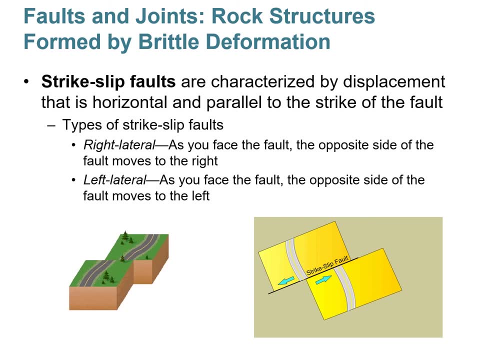 And then these older rocks are being thrust over these younger rocks and essentially you can create a range like that. Okay. Then there are strike slip faults. These are characterized by uh kind of shearing type, uh stress, where you have two blocks kind of sliding side by side one another. 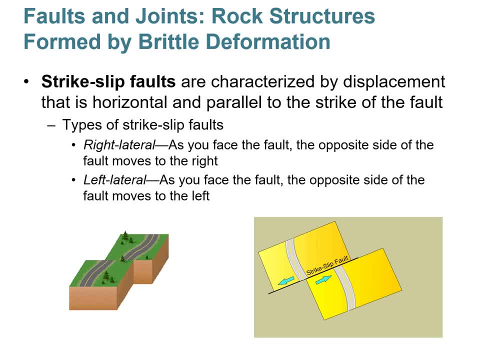 Okay, And there's two types: There's right lateral and then there's left lateral, And the way to figure this out is pretend you're standing on one of the blocks. Okay, So let's pretend we're on this block here and you're looking in this direction. 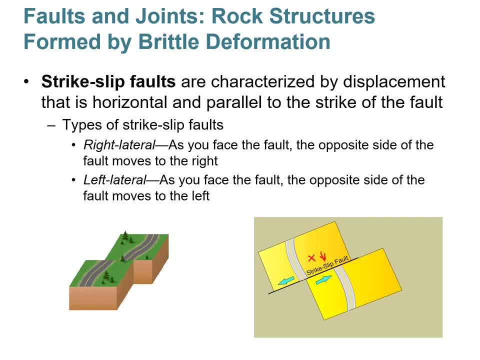 So you're facing this block over here. Um, when you, when you look at that block, which direction Is it moving in? it'd be to your left right. So therefore, this one right here is a left lateral strike slip fault. 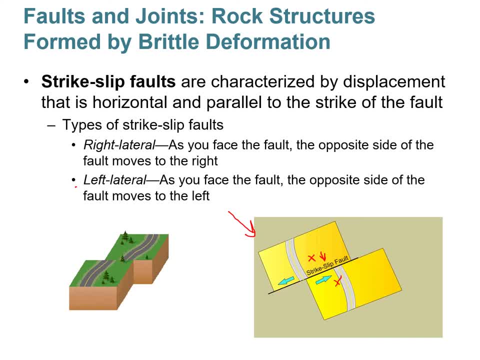 And the same is true as if you're pretending you're standing on this side of the block and looking over the fault at this block, And this block is moving to the left from your vantage point over here, So therefore it's a left lateral strike slip fault over here. on this example, if you're standing here and looking over the fault, this block is. 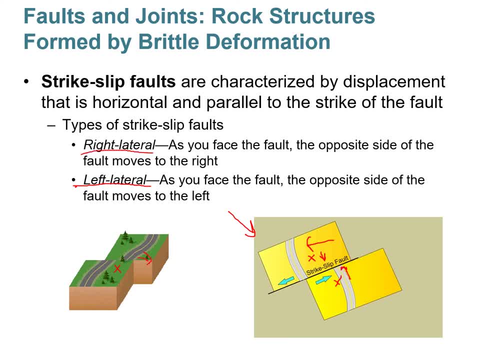 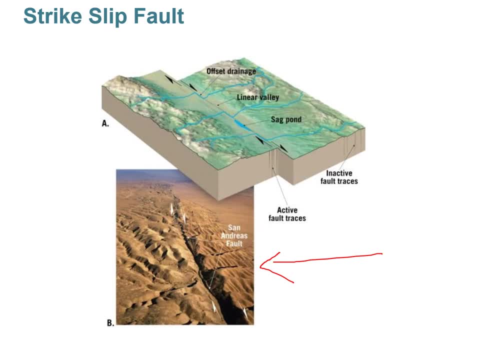 Moving to the right. So this would be a right lateral strike slip fault. Here's another example. here It is in the real world. This is the San Andreas fault. Um, can you tell me what type of fault this is Right? 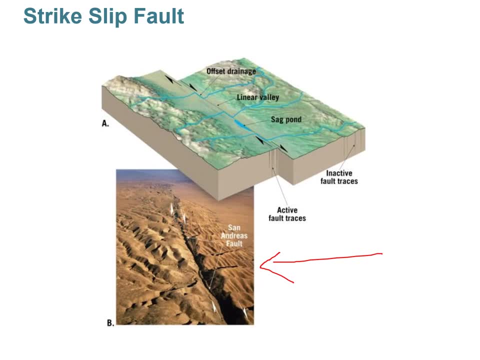 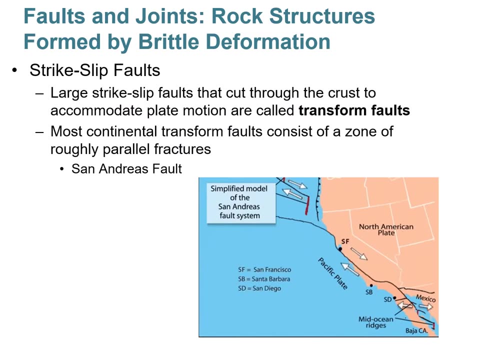 Or left lateral, You are correct, Right Lateral. Nice, Good job. So proud of you. Okay, So you can have a large scale strike. slip faults, Uh, we call those transform faults. They Accommodate uh plate motion, uh, in very large plates. 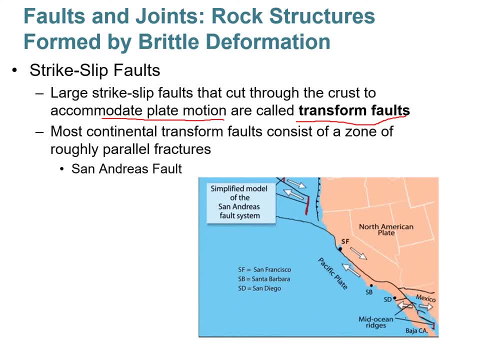 And one cool example is the Pacific plate. Here's a simplified model of what's going on out west and why they have earthquakes. So this portion of California and Baja California here are part of the Pacific plate and they're kind of moving north, uh westward, relative to the North American plate. 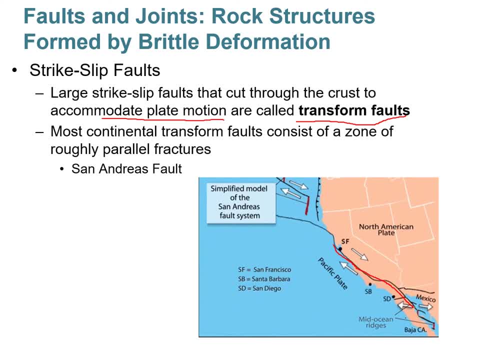 And that's why there's all these earthquakes here And here is the zone of, uh, all those transform faults really is like a zone Of a lot of different faults, that major faults that form here. There's another major one, uh, in New Zealand. 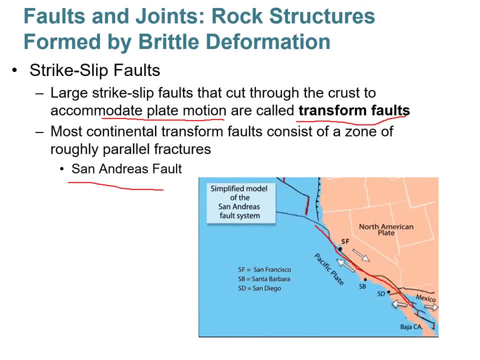 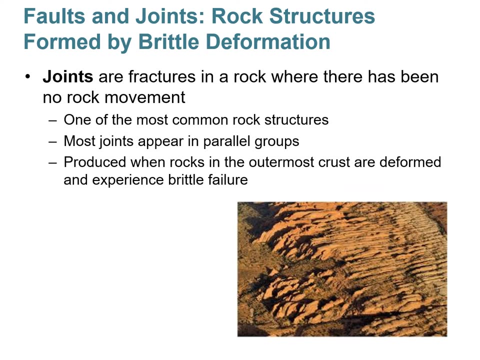 That's why they have a lot of earthquakes there. And then, uh, there's one that goes through kind of um, uh, like the Caribbean part of the Caribbean plate and goes right through Guatemala. Okay, Joints, joints are fractures in a rock, that where there's no movement, but so it's kind of like the rock is expanding and cracking in this parallel fashion. 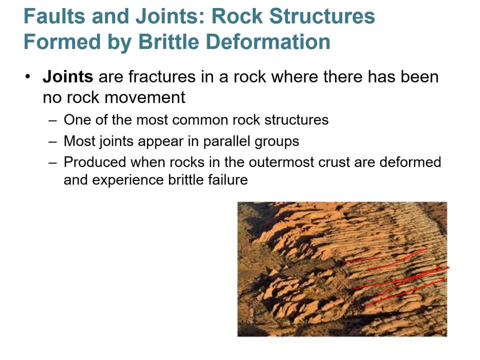 So these are all joint cracks Right Here. see that they they mostly occur in groups. Okay, And so when rocks are at the outermost crust, uh, they'll experience this brittle failure. Okay, All right, Let's shift gears and talk about mountain building. 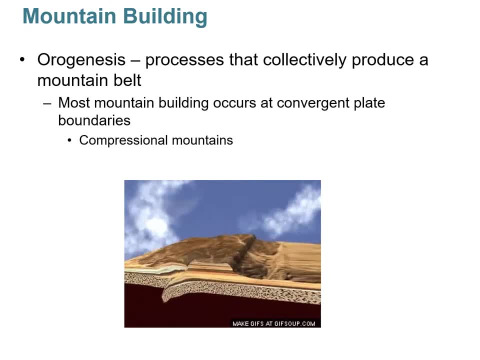 The uh fancy word for mountain building that geologists came up with is called orogenesis, And so, uh, the reason why they came up with this term is because a lot of things can happen in the process of creating mountains, So we kind of give it a blanket term called 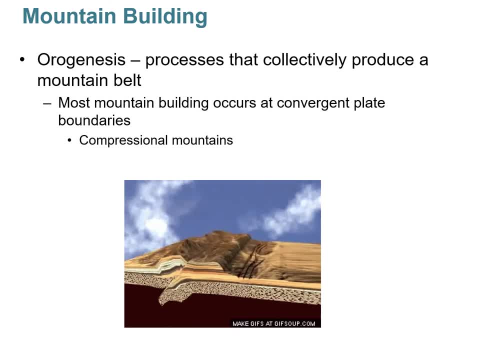 Orogenesis- All the processes that collectively produce mountain belts- is an orogenic event, And so most mountain building occurs at convergent plate boundaries and you create compressional mountains, And that's what you're seeing here. This is a little model showing you how mountains are generated. 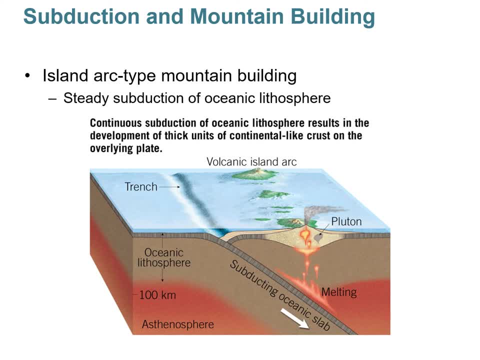 So the first type of mountain building um is associated with subduction, and remember so a subduct, sub subduction zone is a convergent plate boundary And Here you have a steady subduction of ocean lithosphere. right Here's a downgoing ocean plate. uh D waters creates melts and the 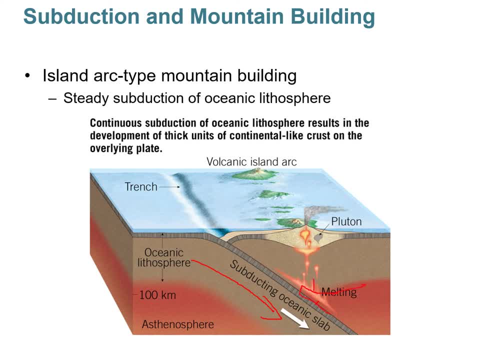 This a Stenispheric mantle. those rise up uh, thicken the overriding uh crust here And some of it erupts at the surface to create kind of a volcanic Island arcs Right And because of this kind of uh collision, this compression, the overriding freight kind of buckles and thickens. 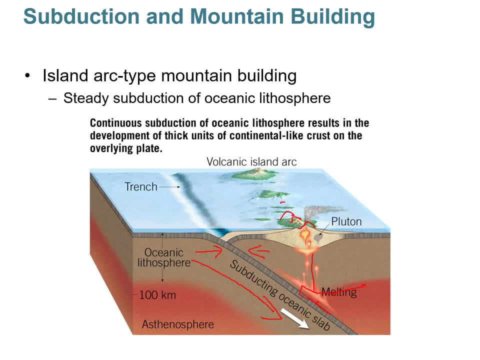 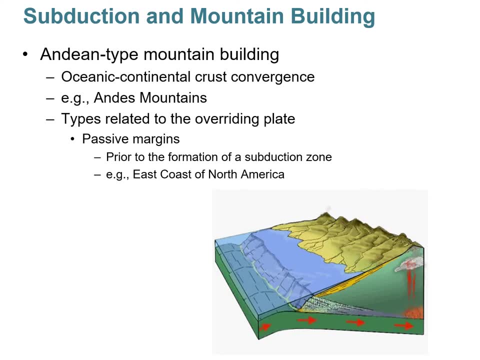 So, Right, Yeah, as a result of it- and that's how you can kind of start the mountain building process here- and if this occurs, occurs over millions and millions of years- this leads to andean type mountain building, and this is where you have ocean and continental crust converging. so you see, here this is the 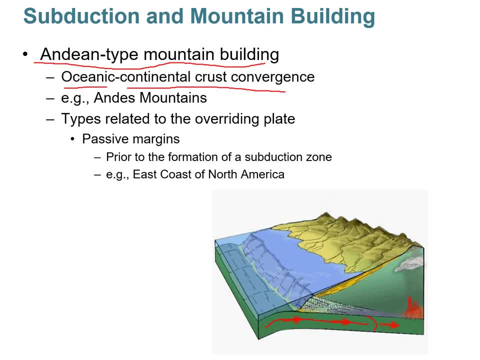 subducting ocean lithosphere. being kind of taken down, melts are generated, this kind of thickens and may erupt at the surface. a lot of them crystallize deep underground as intrusive igneous rocks, but as a result you have mountains like the andes. god, i love how these little volcanoes smoke. 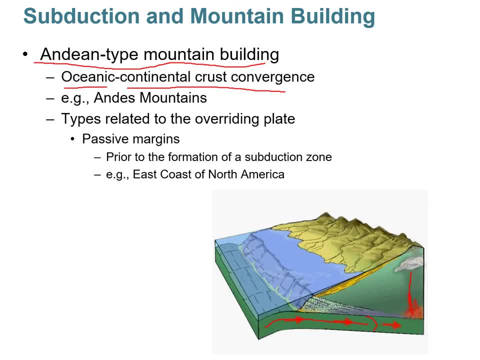 so, yeah, that's, the andes are a majestic mountain chain that divide kind of chile and argentina, and they kind of go through the go through peru, ecuador and colombia, okay, um, and so what happens? the way this kind of it onsets is you start off with a pattern. 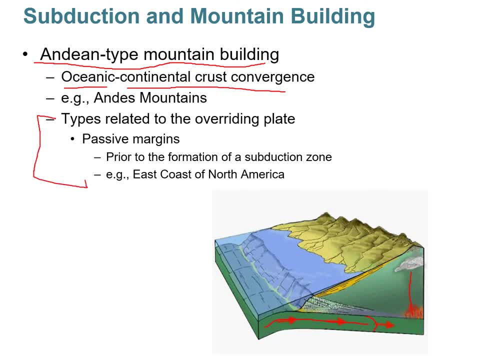 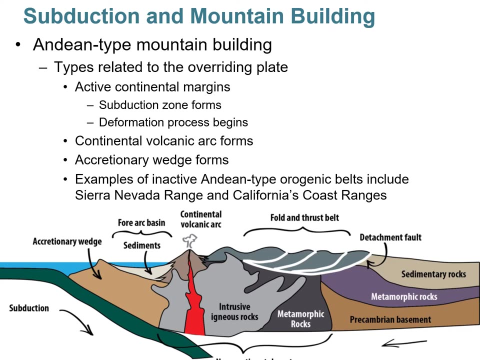 of subduction and then you get the onset of subduction and then continuous subduction for millions of years and that thickens this overriding plate and also pushes these rocks upwards and compresses them, okay. so here's the example, these are the features that will form. here's the: the continental volcanic arc. 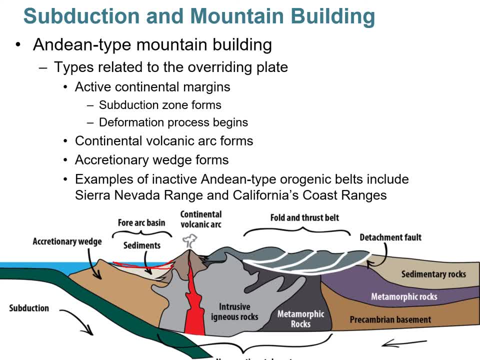 you'll have a four arc base in a low-lying area where a lot of volcanic sediments deposit the formation of an accretionary wedge. here's the subducting plate. the reason why this is there: because a lot of times the ocean sediment. 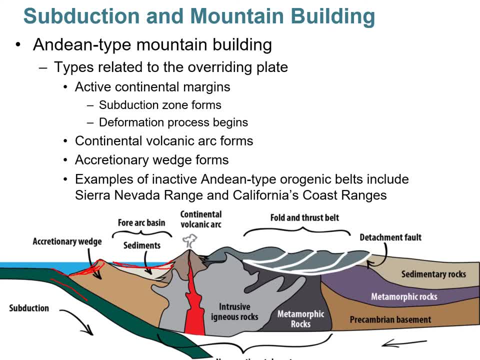 can get kind of plastered on the continent here, a lot of intrusive igneous rocks that leads to metamorphic rocks that are over here and then back here is where you have the fold and thrust belt of mountains. okay, so you have the continental volcanic arc form. that's this area. 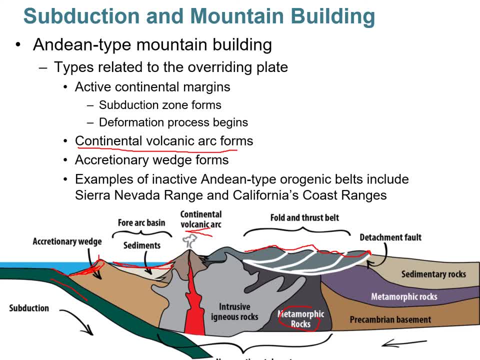 the accretionary wedge form and then, uh, and then here are the andes just west of the- um, i'm sorry, of the volcanic chain, let's say, let's say the andes in as an example. other, uh, inactive examples are the sierra nevadas in california, and california's coastal ranges were the result of. 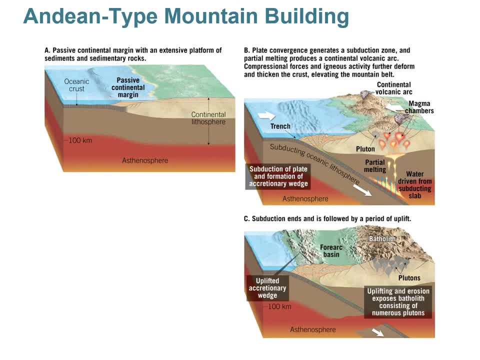 andean type mountain building. okay, so here's, here's that process. you start off with the passive margin. right, there's no subduction here. it's far away from plate boundaries. but then there's the onset of subduction, subducting ocean lithosphere. here's the trench, this is the accretionary wedge starting. 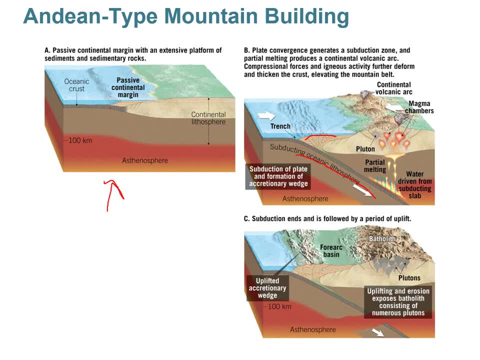 to form, and then there's the subduction of the ocean lithosphere. here's the trench. this is the accretionary wedge starting to form, and then you're starting to create your continental volcanic arc. the crust is thickening, those thrust faults start to form and then you get a mountain. 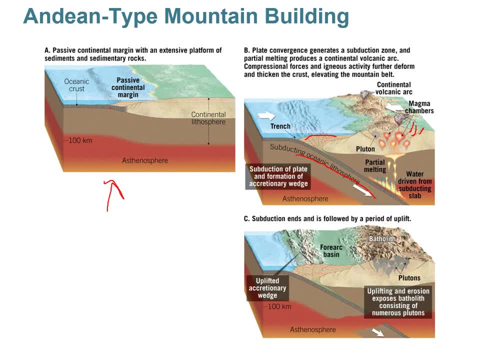 chain, like you see here, and this is basically what california essentially looks like. this is. these are the sierra nevada mountains, where yosemite national park is and there's a central valley in california, and then the coastal mountains here. this used to be a former accretionary wedge. okay, then there is a collisional mountain. 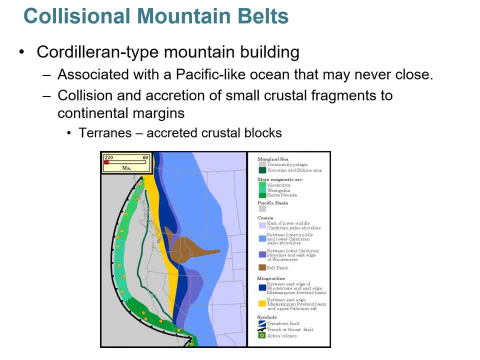 and this is a kind of more complex mountain building um, and it's associated with like uh, like uh pacific, like ocean um uh, basins that are kind of like uh closing, essentially, and island arcs or microcontinents collide with larger continental crust and so this process 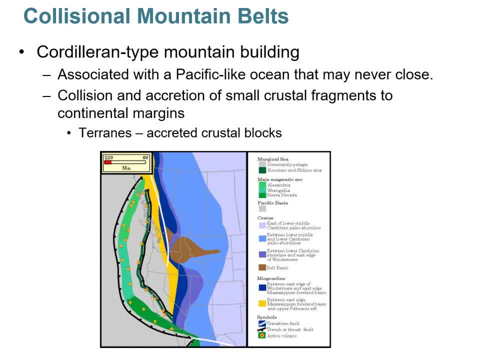 creates, um, like accretion of those small crustal fragments that you think are very well known, like you know, at the oak richards or where there used to be maybe island arcs or ocean plateaus or microcontinents, and that stuff gets plastered onto the continent when we call those terrains or exotic terrains, because they didn't really. 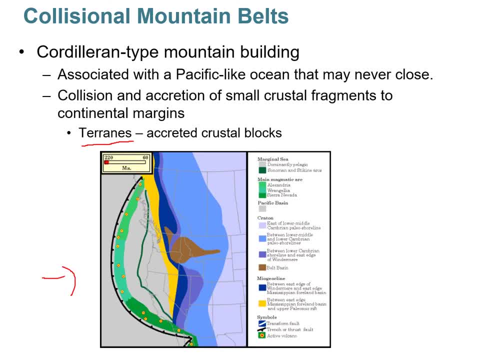 like belong to the continental crust and they were just kind of added to it and you can see that in this gif here over the course of let's see 200 and or 180 million years continued subduction here and ocean provinces and microcontinents and islands and continent- uh that stuff- are pretty nice. 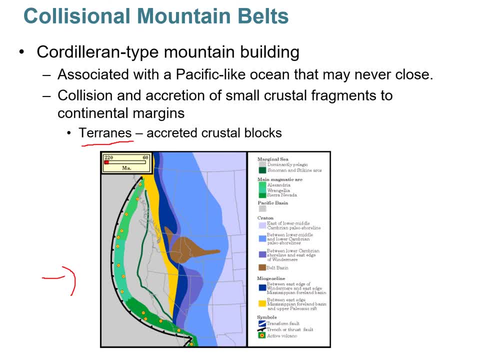 the continental crust and those are the agricultural cork crusts. these are the organic crusts and they're mostly strong and they're not on top of the other one until they're alive and then they're just kind of continents, and island arcs were kind of added to the western side of North. 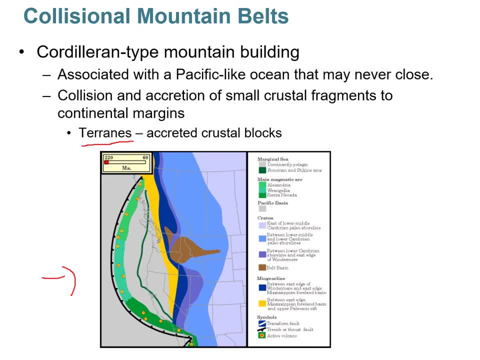 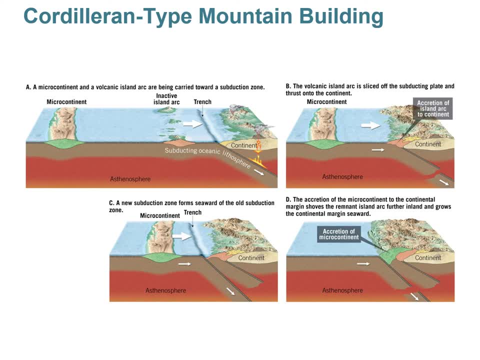 America, And each one of these different colors represents different terrains that were added to the continent. This might make more sense here. So if you have a subducting ocean lithosphere, pretend this is the west coast of the United States. So here's the continental volcanic arc and, as you 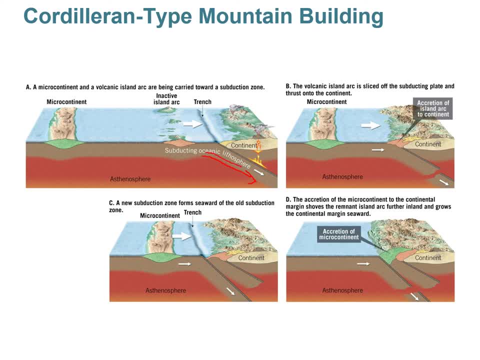 subduct this ocean plate. here is an inactive island arc, So think of, like Japan or something, A couple islands. This stuff is really buoyant and won't subduct with the down-going ocean plate. So what will happen? is it just kind of? 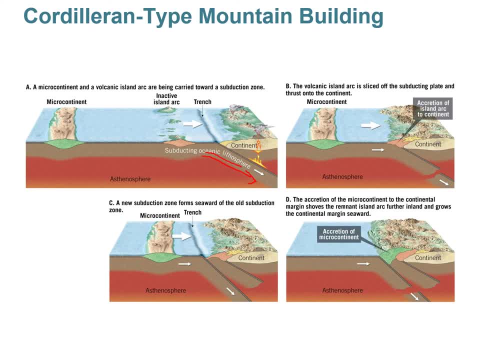 plasters itself and becomes part of the overriding plate. So you see that You can see this kind of yellow color here. That's the material that just got added to it. So an island arc added to it And then you can have something like a. 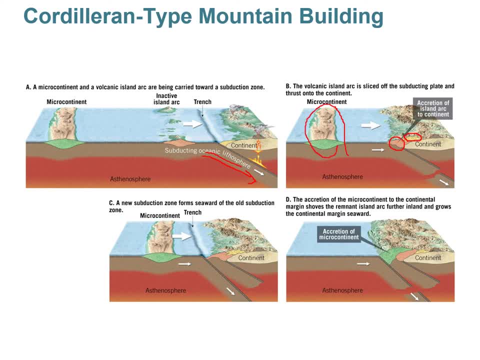 microcontinent, Let's say like a Madagascar or something, That will approach the subduction zone and it won't subduct, So it'll just get added piecemeal To the existing crust over here. And this happens repeatedly, over and over again. 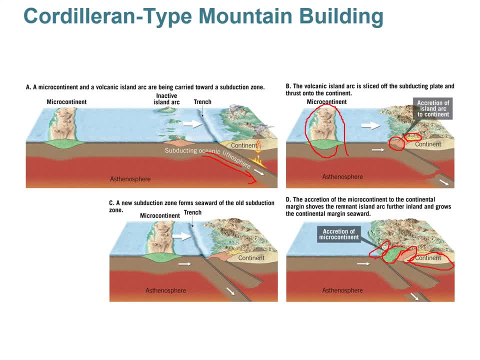 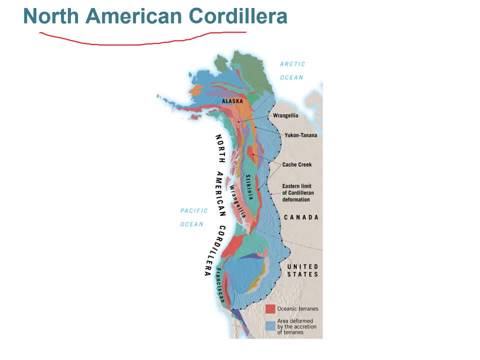 And then what you get is a bunch of exotic terrains just kind of piled up on top of each other, And that's the case of the North American cordillera. This goes from California all the way to the tip of Alaska. All these different colors that. 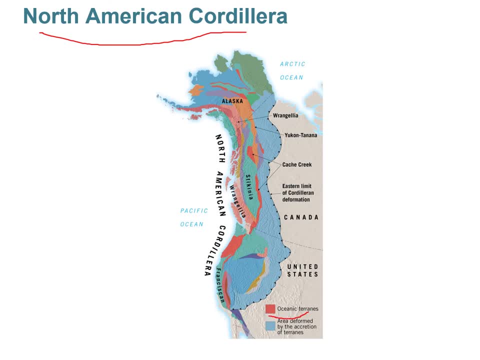 you see are different: either oceanic terrains or former microcontinents or island arcs that have been added to the west coast, that are in the university, and the south coast. It's actually very complex geology. They are very complex and complex geological And you know that. 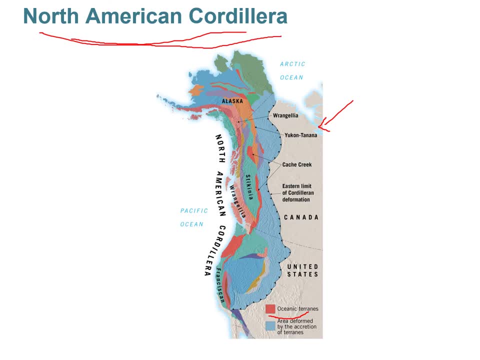 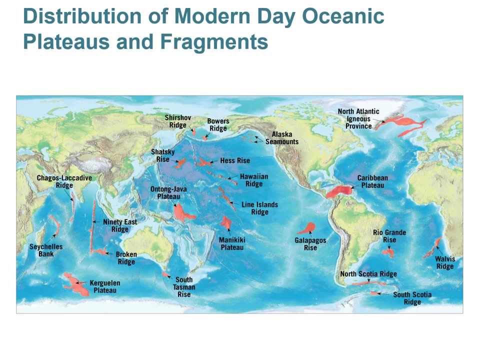 the continent is very complex. You have something like the Kảiland. It has a very complex geological structure. It has a very complex geological structure, Tectonic plate Right, So that's why we refer to it as kind of cordillera and type mountain building Very complex. 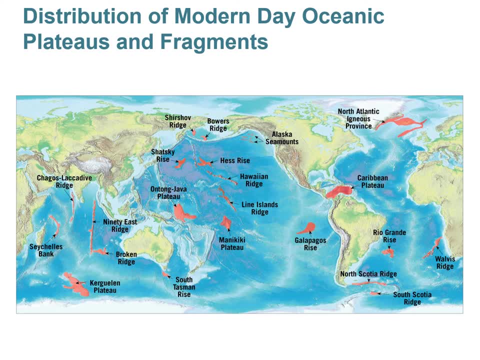 geology. If you go out here, it's complex because these are very old deformed rocks. they've been through a lot onto continental lithosphere, if subduction kind of continues and and so basically these could be the new terrains or exotic terrains that have. 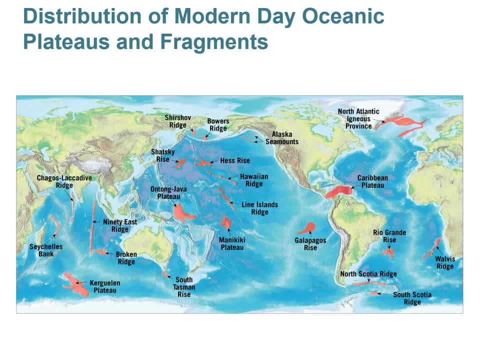 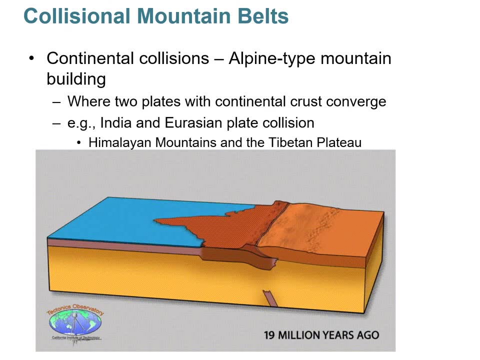 been that could add on to continents, and the idea is here is that's how a lot of kind of crust must have formed initially is through this process of subduction, okay. the last type of mountain building is called collisional mountain belts, or these huge continental collisions. we call these alpine type mountain building. 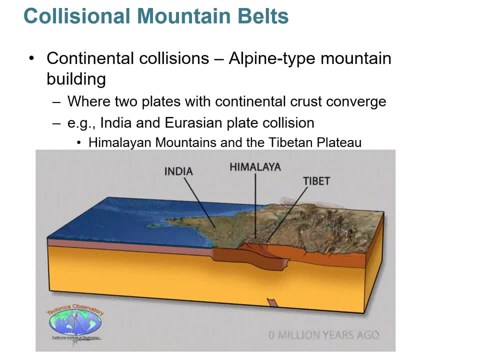 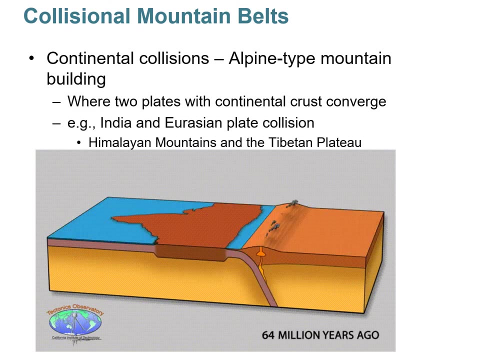 were to continental crust tech, like plates kind of collide okay, and the best example of this is the Alps or the Himalayan mountains. here this is the past 60 million years. India was kind of its own island, island in the middle of the world, and it was kind of the first continent in the 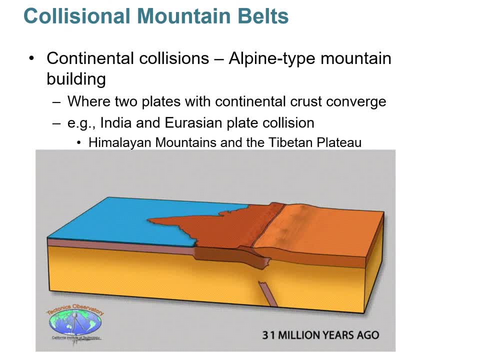 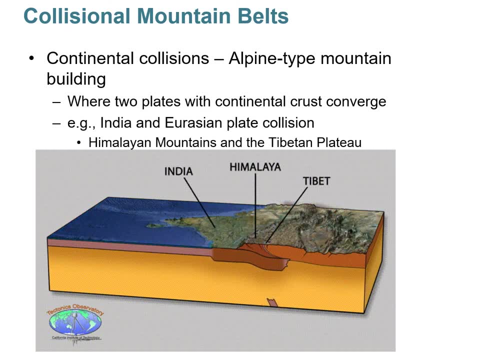 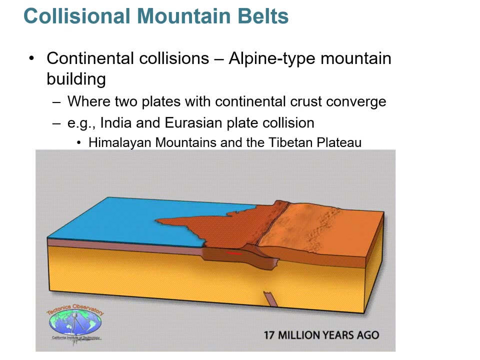 continent and it slammed into Eurasia and as it did there was, it had a leading edge of a subducting plate, but it kind of ran out of that subducting plate. so initially there was a continental volcanic arc in Eurasia- you see that here- but then as a subducting plate kind of tapered off, then it was continental. 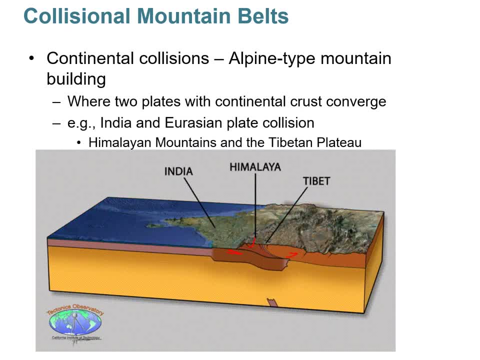 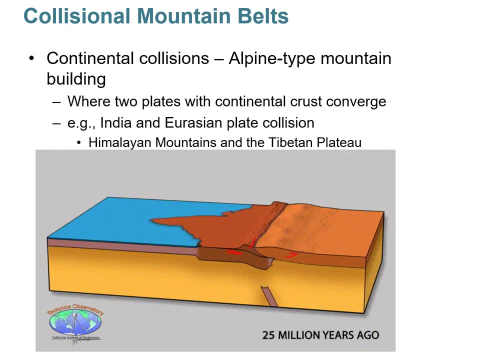 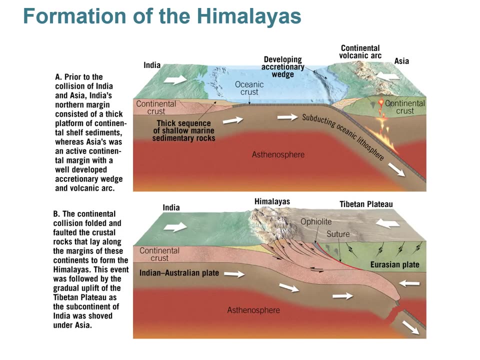 crust on continental crust and that's what is pushing up all those crustal rocks upwards and creating those majestic Himalayan mountains. that's a great gif. Okay, so here's just another image of that. so initially, here's India. this was the subducting ocean lithosphere. you. 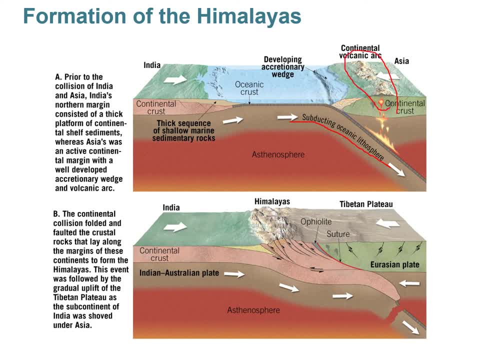 had a continental volcanic arc. all right, there were some kind of mountains here as a result of that continental arc volcanism. you could even say that this was kind of like pre Indian type mountain building before India just slammed into the Eurasian continent and that's what formed a rough mountain. 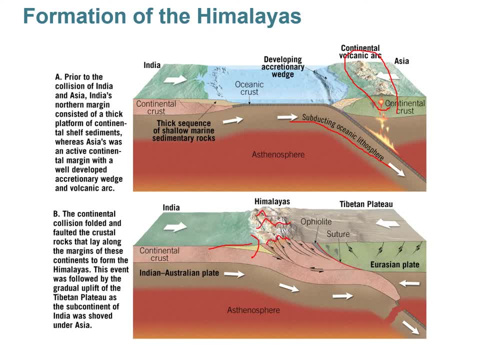 We did that 5,000 years ago- formed what the Himalayas are today: the the largest mountain chain and the highest mountain chain still growing. I mean, India is still kind of pushing northward into the Eurasian plate, and then there are the Appalachian Mountains. 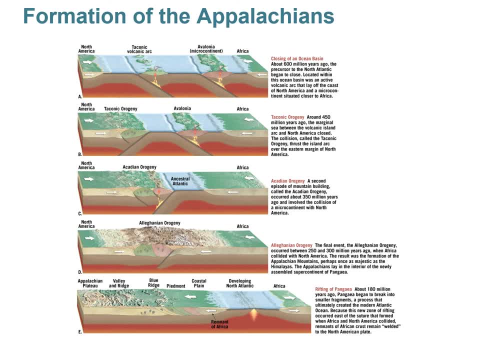 the Appalachian Mountains are much older and they kind of record all kinds of crazy tectonic history. but if you go back 600 million years ago, here's the North American plate. there was a volcanic arc here in an ancient ocean before the Atlantic Ocean. then there was a microcontinent over here and then here. 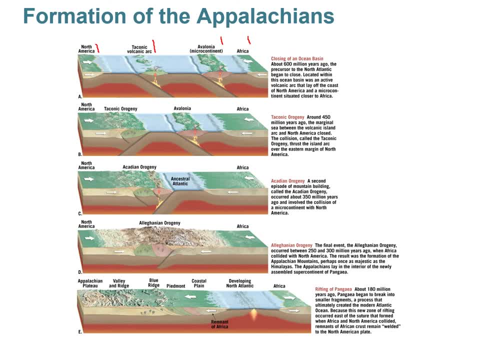 was the African continent. so the first step that occurred was the tectonic orogeny. so here, this exotic terrain, this volcanic arc, was added to the North American tectonic plate. okay, then, over the course of the next hundred million years, Avalonio, which was its own microcontinent, then slammed into the 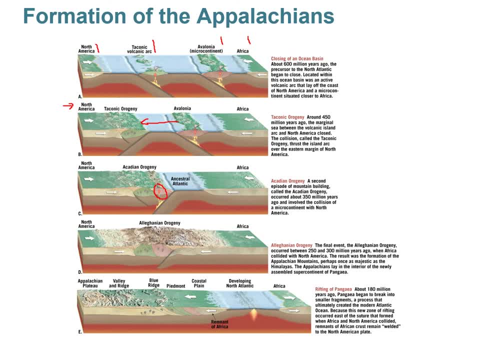 North American continent and that added another exotic terrain to the North American continent and then this is the ancestral Atlantic, it's called the Iapetus ocean. and then Africa came in and then slammed into North America and this was the kind of culmination and the building of the Appalachian Mountains in. 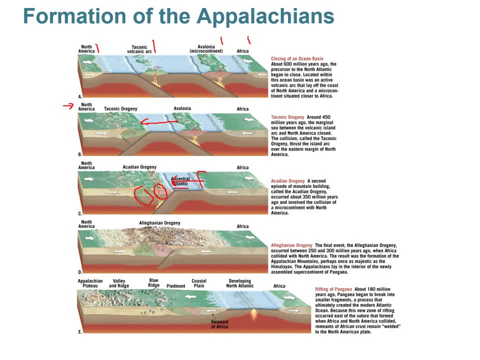 its totality. okay, and at this time, about 250 to 300 million years ago, the A hurérieur surface was in the 6th century. as compared to the Apalachian Mountains, rivaled the Himalayas of today. okay, since this time it's been 3. 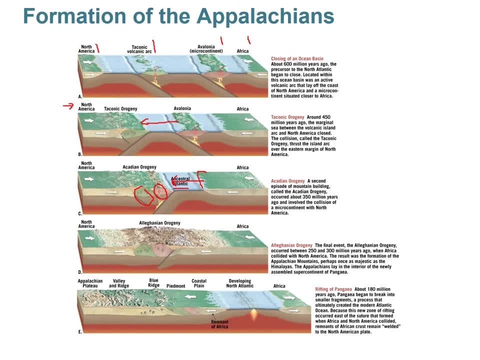 300 million years of slow erosion and it's kind of rounded off a lot. and it's kind of rounded off a lot of the of the exposed rocks here. but oh yeah, this was in the time of Pangea as well, so it is in the Tanaherts around. 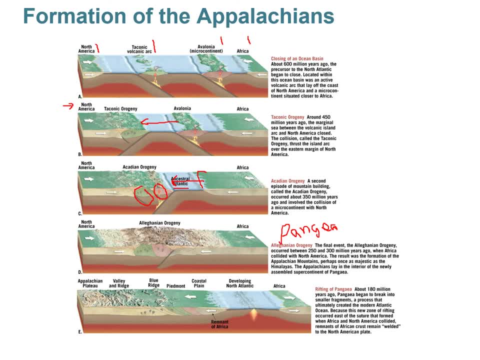 this long ago and this was a major mountain chain. so since then Pangea Kekkaafranjietvi broke apart and found a rock out west, so thisttles is the third island. this is another island effectively raveling city rock cliff that we just went down calmly. we don't have once in沒 espenerad. 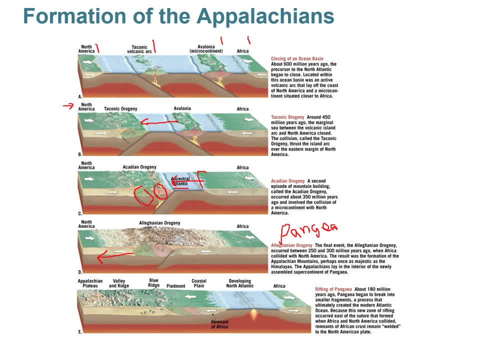 then Pangea broke apart Africa and there was a continental rift and the rift kind of formed over on the kind of African continental side and so actually a piece or remnant of Africa is still attached to the North American plate. and guess where that remnant is? yeah, Florida, Florida, if you dig deep enough past the. 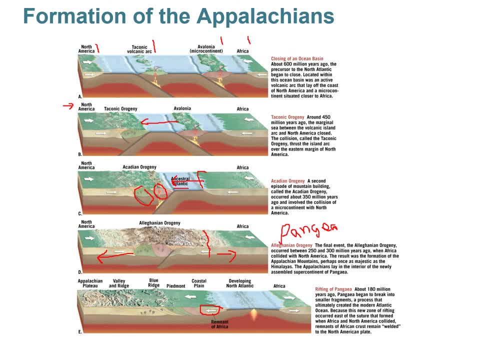 like 10,000 feet of limestone. you get down to African metamorphic basement and that incredible. so we were once part of Africa and we rifted off. we ripped off of that lithosphere back when Pangea broke apart and now we're the remnant of 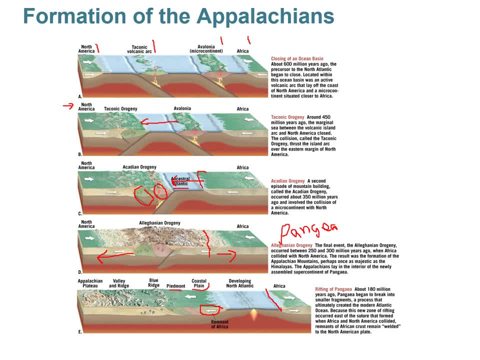 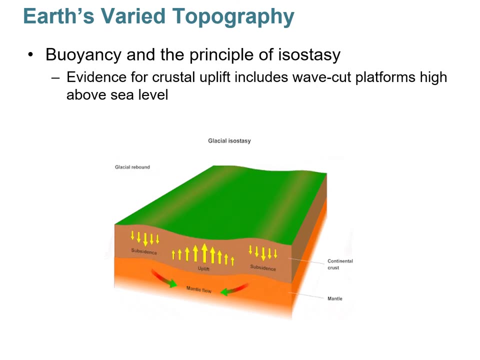 it as part of the coastal plain in the United States. and then these are the different physiographic regions: the Blue Ridge Mountains, Piedmont, and then the valley and ridge province behind the Blue Ridge Mountains. so that's the story of the Appalachian Mountains. okay, so let's talk about the. 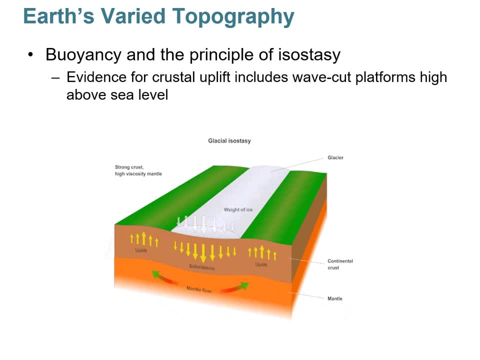 you. principle of isostasy and buoyancy. okay, there is evidence that there is crustal uplift, meaning like the crust rises upward above sea level because of features that the ocean will create, like the. the ocean will will erode continental margins and create wave cut platforms that are very flat, but in a lot of 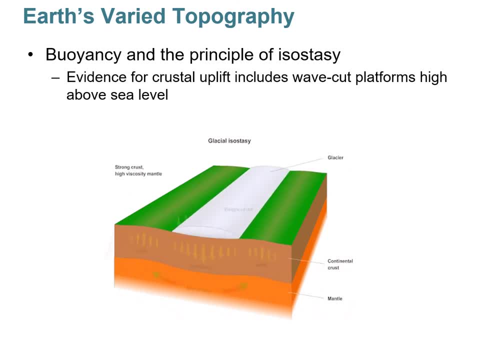 areas we can see multiple wave cut platforms above sea level. so there's evidence that in certain areas, maybe because of plate tectonics, there's crustal uplift. but there's also another example of where crust can be uplifted and that's the process of isostasy. and in this example, this gif, it's going too. 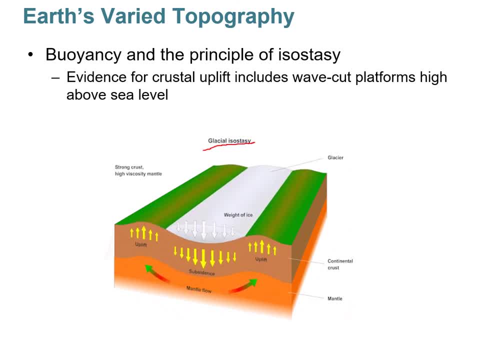 fast, but this is example of glacial isostasy. so up is there. what is the main part of this tattoo? that thisriel Phew construction? it just has to do loads満. but when the weather, when climate changes and we're in an interglacial, 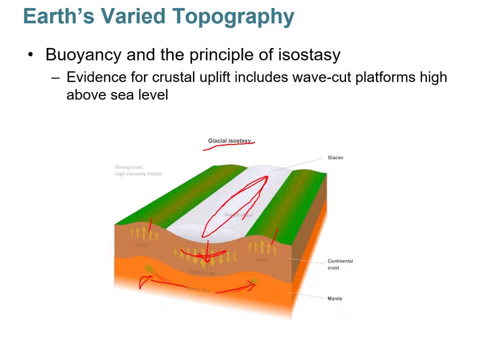 period. this: these glaciers melt away and as they melt away, the weight of all that stuff is removed from the crust and the crust actually kind of rebounds and rises, and that's true in places like Norway, like right now. sea level is rising millimeters every year really slowly. so globally continental margins: 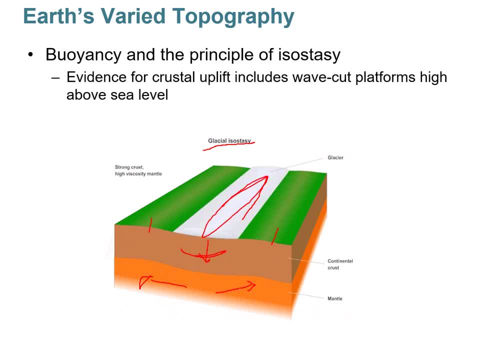 are seeing sea level rise, okay, but in Norway they're actually seeing local sea level fall because the rate of crustal uplift is faster than the rate of sea level rise. so they're seeing sea level fall in their perspective and that's just because the crust is rising faster. 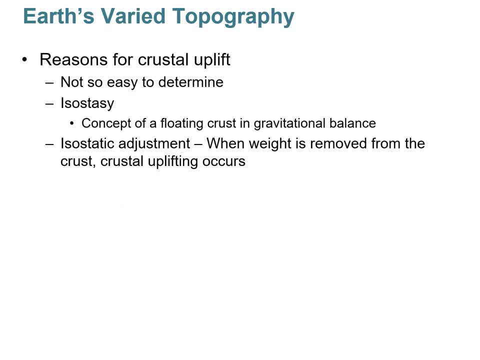 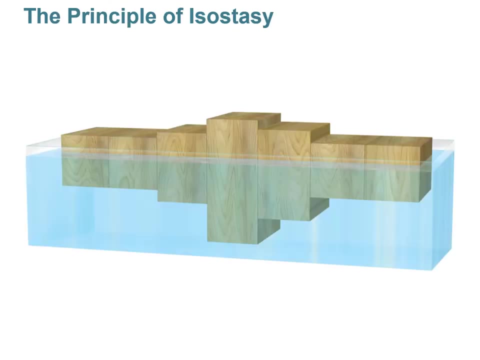 and so the way to understand isosceles, just to imagine floating crust that's in gravitational balance and then when you have subsidence or uplifting, that's an isostatic adjustment. okay, the book is an example of floating blocks. I prefer imagine you ever see those container ships that carry those like 40-foot. 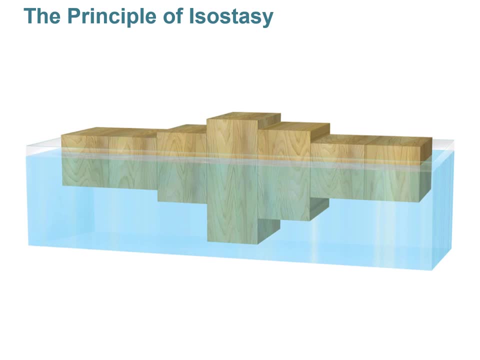 containers that go into ports. right, just imagine this. right, imagine one that's fully loaded, fully loaded, and as you remove those containers one by one and you empty one of those boats, what's that boat gonna do in the water? right, it's going to rise. right, it's gonna rise up as you remove that cargo. and likewise, if 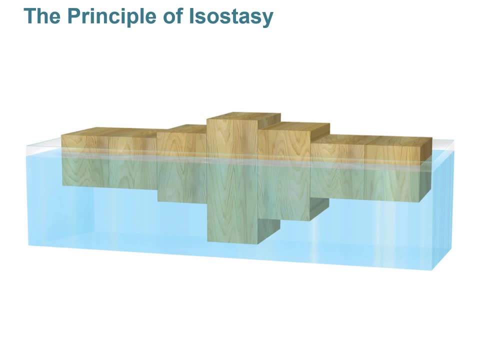 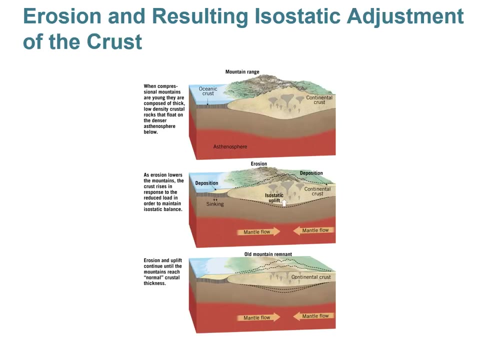 you put cargo back onto the boat, the boat's gonna sink into the water because it becomes heavier. the same thing occurs with the crust. okay, and the same thing occurs. you have mountain building events. when you have mountain building events, you're piling up, piling up all those cargoes and then, as you remove those,